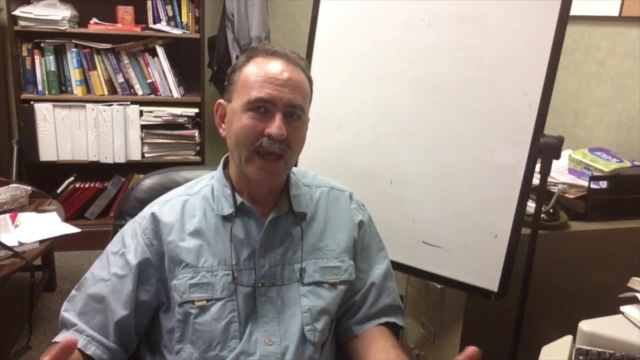 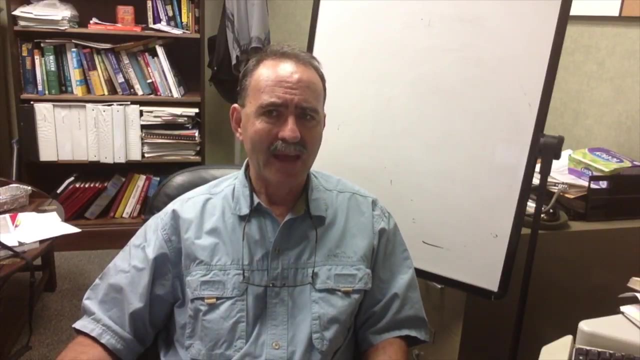 That's when we know that there are soils that are classified as soil taxonomies. So when we know what kind of a soil we are looking at, from that soil survey we can deduce properties of that soil based on what its name is. So that's extremely useful and important. There are some caveats that I'll talk about when we look at the soil survey itself. 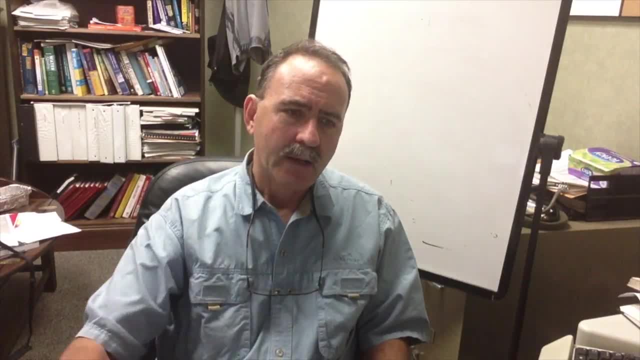 But for now let's go ahead and have a look, Just going back. it's really useful when you want to know something, But for now let's go ahead and have a look, Just going back. it's really useful when you want to know something. 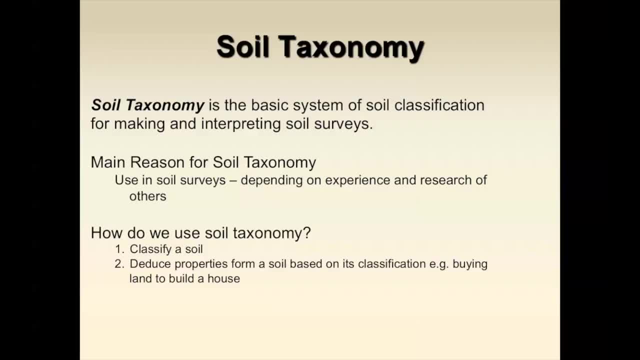 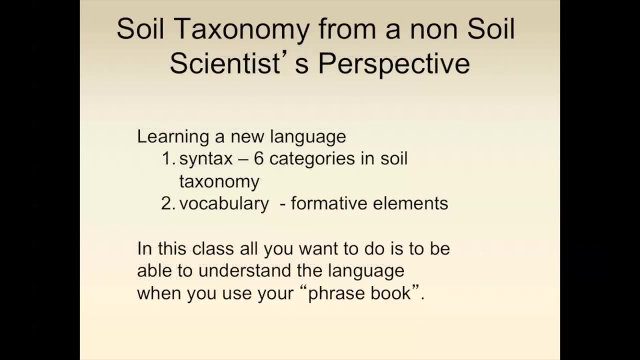 useful when you want to buy a piece of land, whether it's for a house or, you know, for cultivating or whatever it is. you're able to know an awful lot of what, what you're letting yourself into when you understand what the soil is. we're going to look at soil taxonomy from a non-soil scientist's. 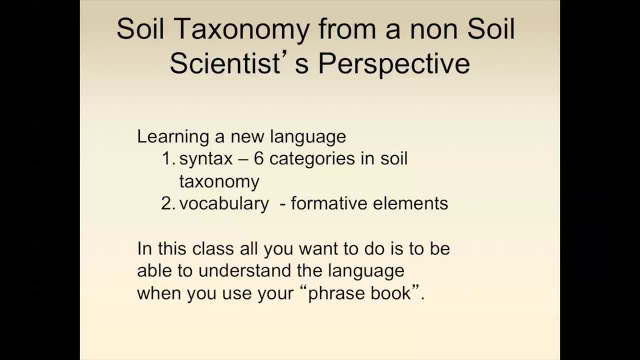 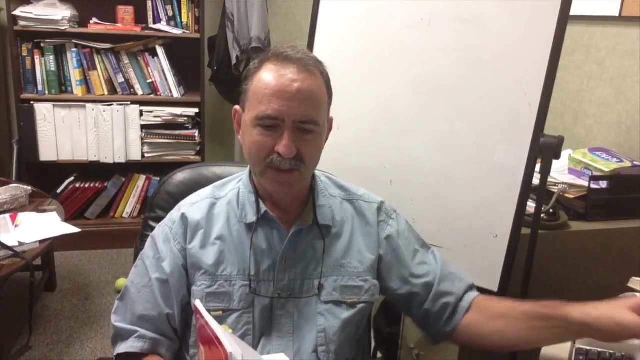 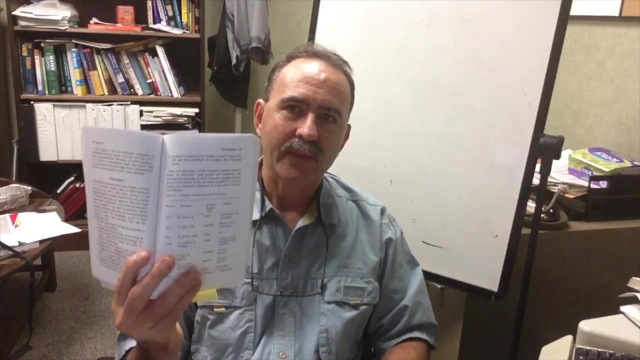 perspective. it's like learning a new language and the syntax, if you will. that is simply the six categories in soil taxonomy. the vocabulary that you have are those formative elements and you will see a number of them in conker and franz meyer chapter 10, and the formative elements are: 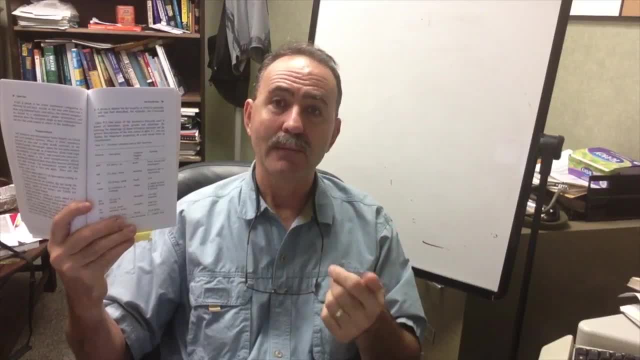 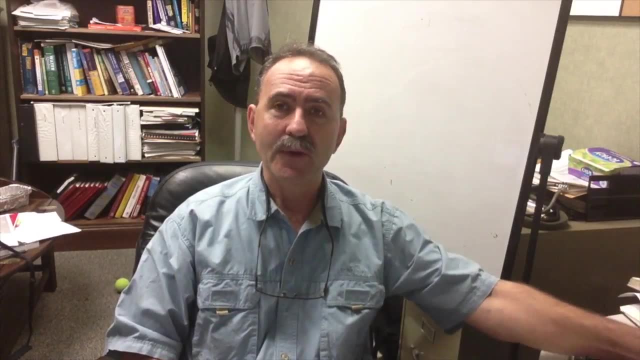 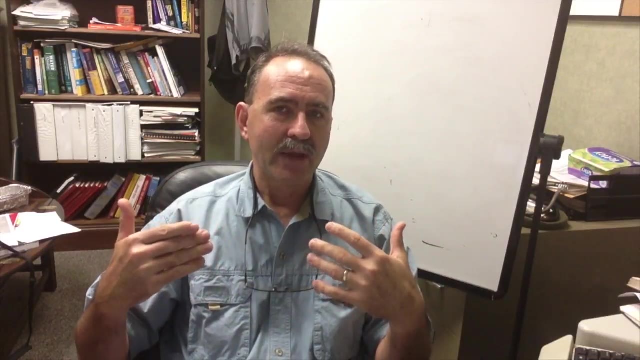 usually syllables that have a certain meaning or sometimes no meaning at all. now I've added a few of those formative elements in here and that should give you enough firepower at least to understand what soil scientists are saying. but when you're reading a book or reading a journal article or talking to a soil scientist, 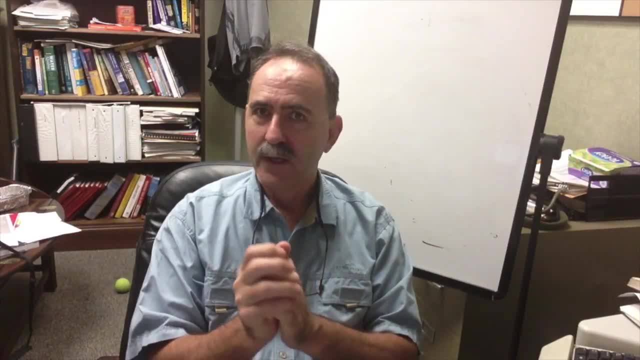 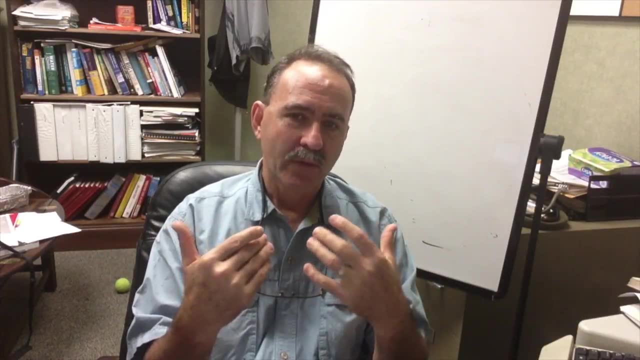 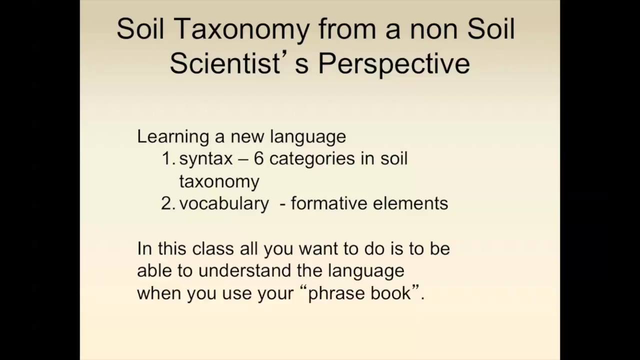 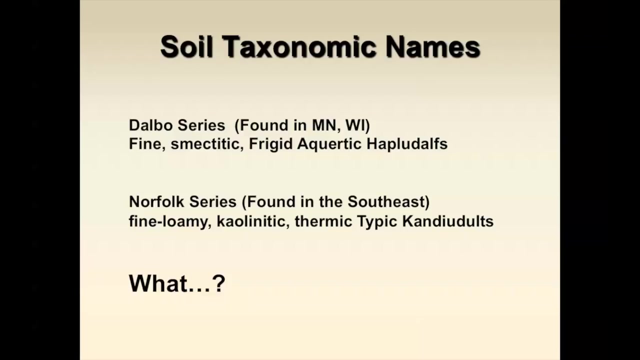 you want to go back to your phrasebook, if you will, to be able to understand what that book or journal article of soil scientists are saying. and you will then be able to understand from that common soil classification some of the properties of that soil, so soil taxonomic names. when you first see it, it's what is this, what is this about? 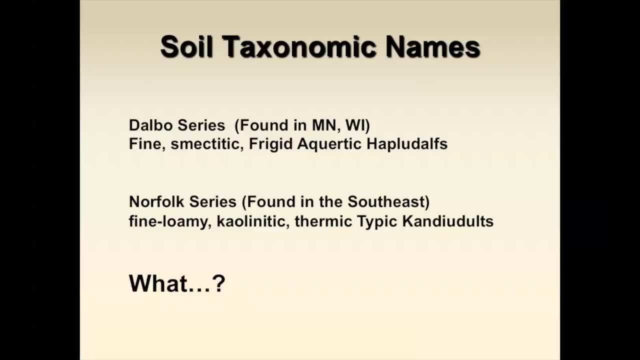 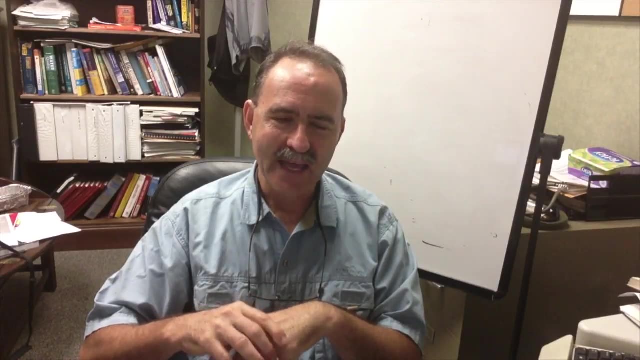 and so let's take a series called the delbo series we find up in the north. it's a fine, smectitic, frigid, awkward, aquatic, happy adult, haplodolph. so if you look at that it's like what, what? what are they saying um the norfolk series which we find down, uh, in this part? 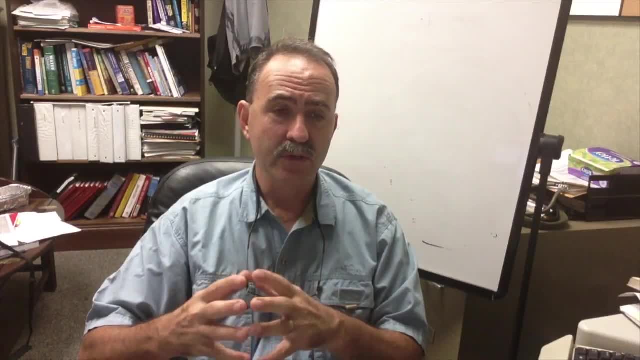 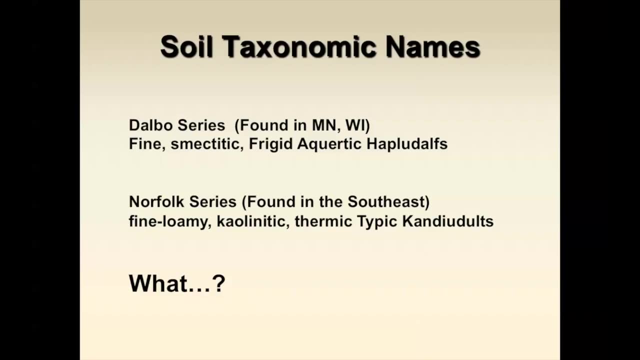 of the world, all the way up the coast to virginia. uh, it's, uh, it's a fine, loamy, kaolinitic, thermic, typic candy udalt. so again, it's what? what kind of you know what kind of crazy naming is this, the? the objective of today's talk really is to kind of walk you through the story of the soil. 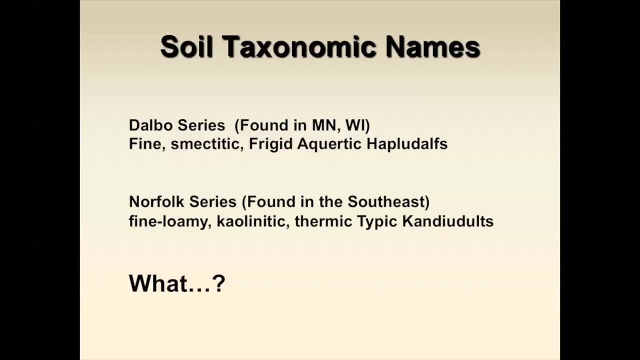 taxonomy and then to kind of go through the nomenclature of these things, so that when i say, or when you encounter something like that, you'll be able to say, okay, i don't know exactly what it means, but i know where to look it up and i know then how to deduce some of those characteristics. 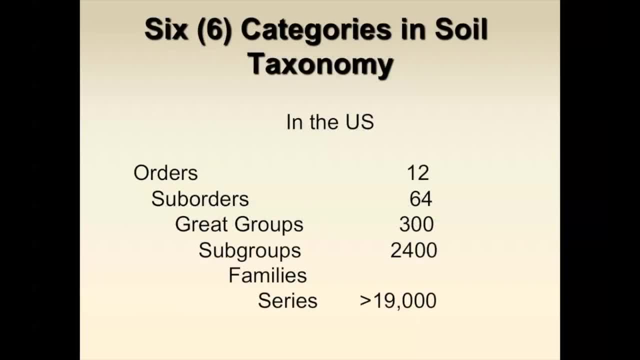 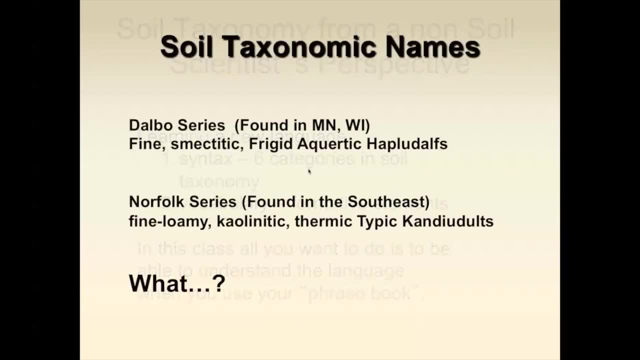 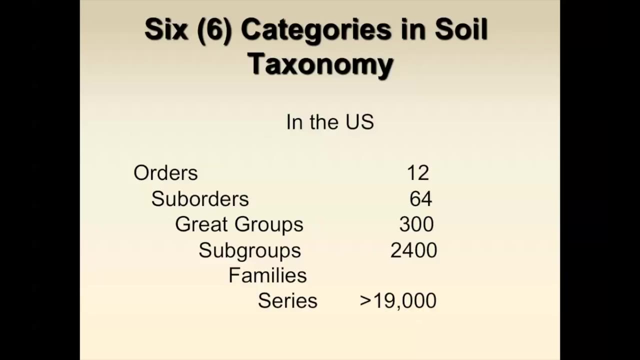 right, let's go back. remember what i said. your syntax over here is that there's six categories in the soil taxonomy. let's go to those six categories. in the united states we have 12 soil orders, or 12 orders, 64 sub orders, 300 great groups. 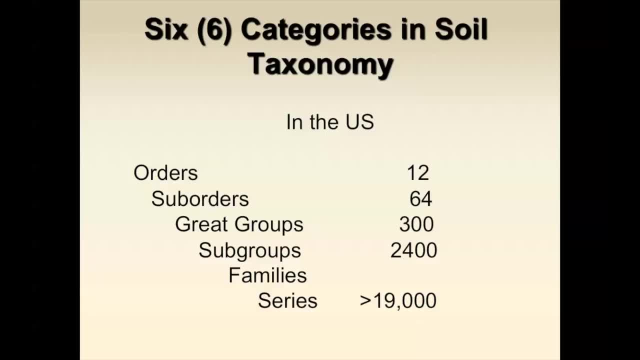 2400 subgroups and somewhere between 2400 and about 10 000 families and then something like 19 000 soil series. so in the previous slide you saw a delbo or a norfolk. those are soil series typically named after the towns or places that they were first discovered. so 19 000 soil series. 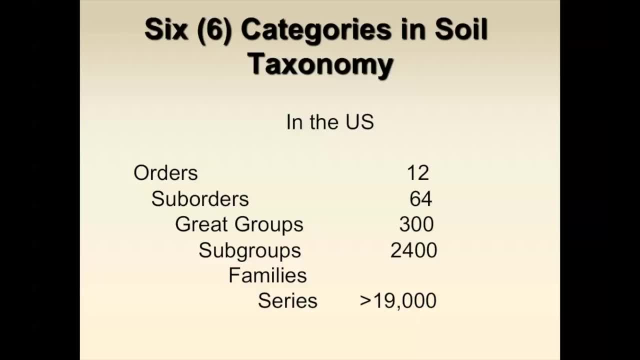 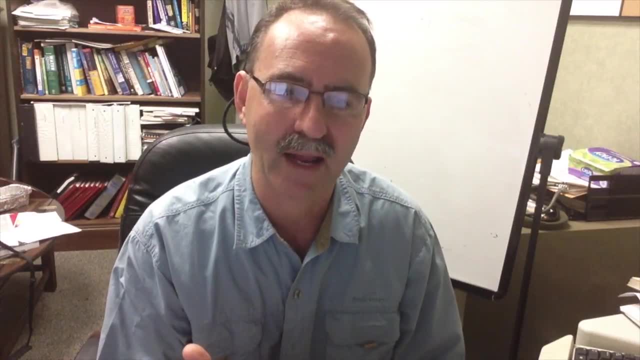 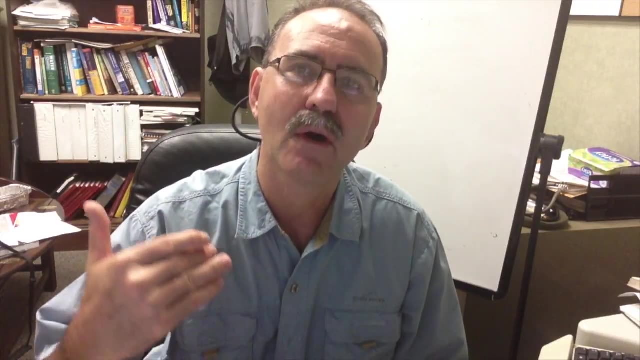 in the united states is is a huge amount and each one of those soil series really is a soil that that looks. if you saw a norfolk in south carolina and a norfolk in north carolina or virginia, you'd be able to say these are some of the common qualities that those soils will have. so let's go. 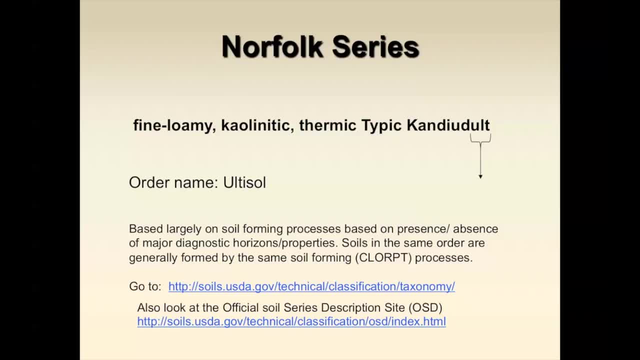 ahead and have a look and take the norfolk series as an example of how to kind of unpack this nomenclature. um, the norfolk series is a fine loamy, kinetic, thermic, typic candy udelt. so if we look at our syntax, our syntax actually starts at the end and it starts with this syllable alt u-l-t. so 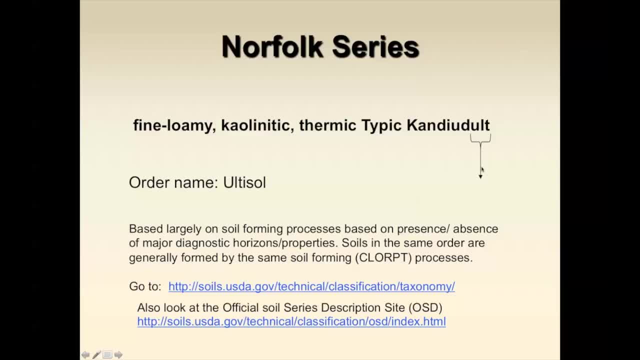 what does that mean? that alt actually is related to the order name. remember there are 12 orders in the in in the united states that is related to the order name altosol. you see those first three letters. altosol is part of that candy udelt. okay, so soil orders, uh, soil order nomenclature is: 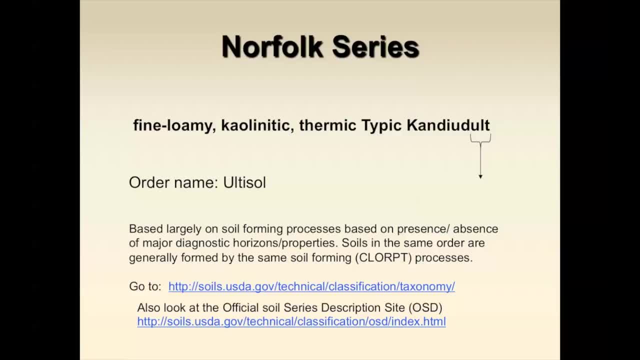 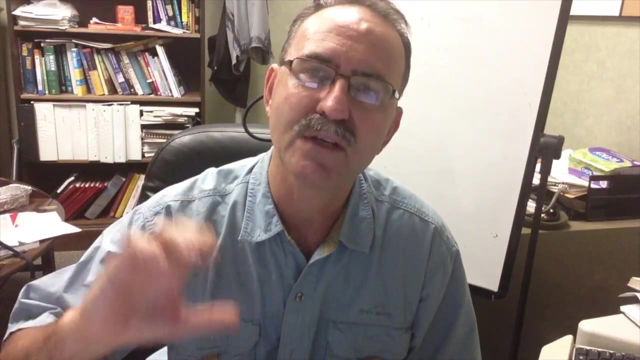 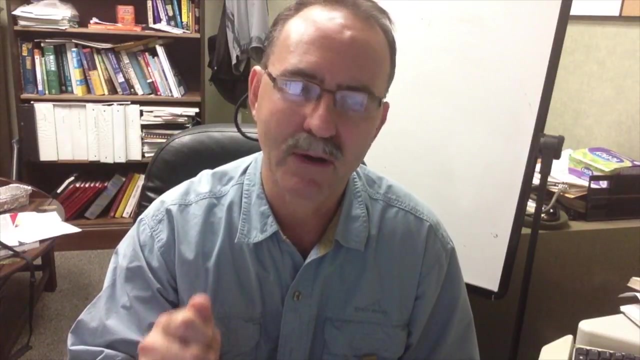 based largely um on the soil form forming processes and the presence or absence of major diagnostic horizons or soil properties. in other words, then there's something very distinctive in one of those soil horizons that's going to give that soil a very distinctive property. i'm going to just very briefly show you. there are two resources. 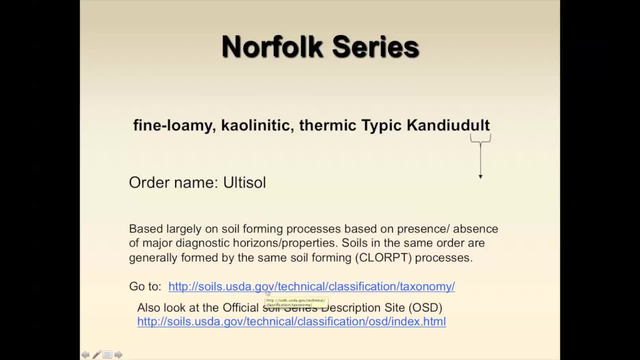 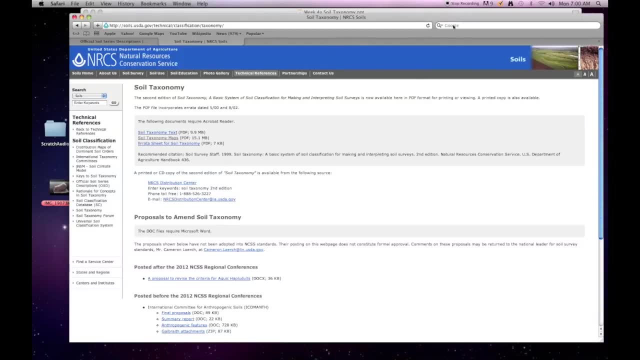 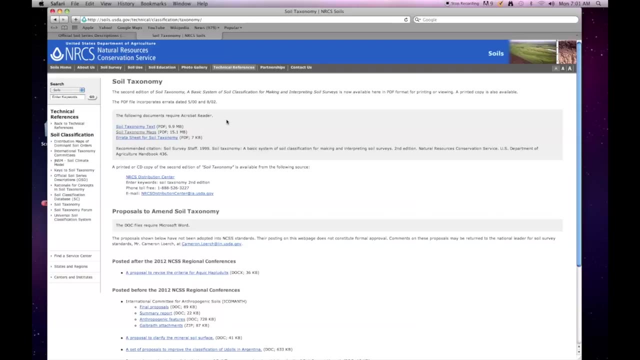 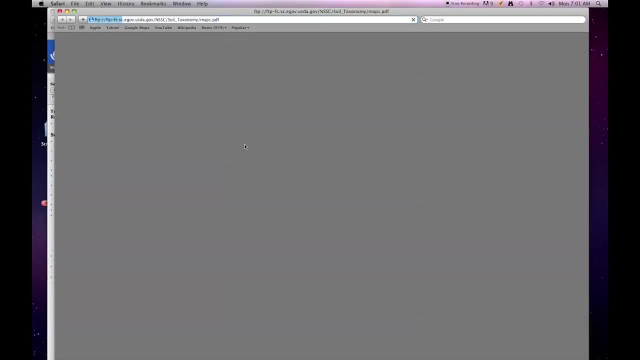 that the usda gives us the soil usda soil survey. i'm going to just back out of this for a moment, and the first is just um a whole, a whole soil taxonomy web page. for instance, there's a text that's about 800 pages, but there's soil taxonomy maps that you can look at. 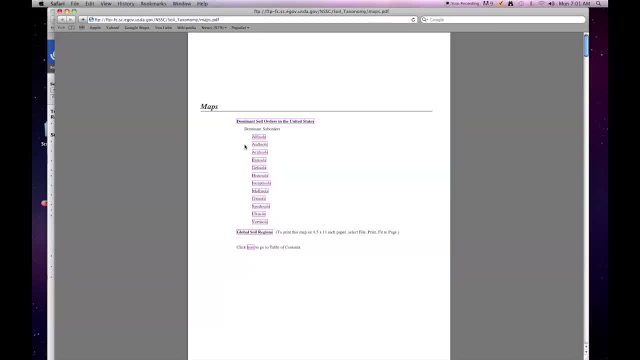 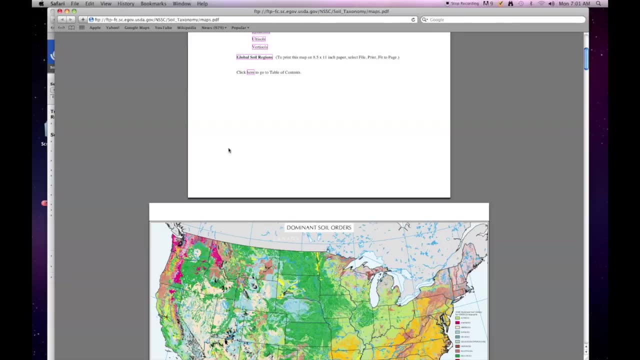 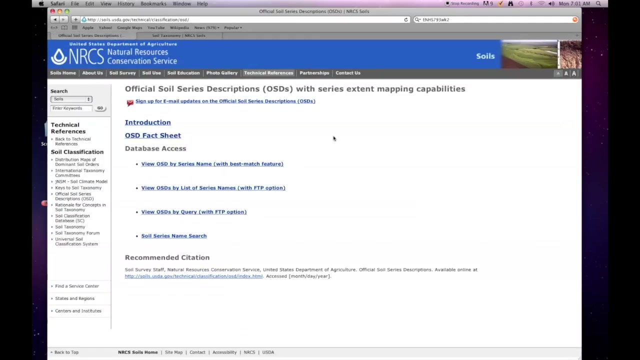 if that interests you at all or if you want to sort of dig deeper into it. so we've got this map. it gives a number of different resources if, if you are so interested in that, the official soil series description. i like this quite quite a bit because i can search, for instance, 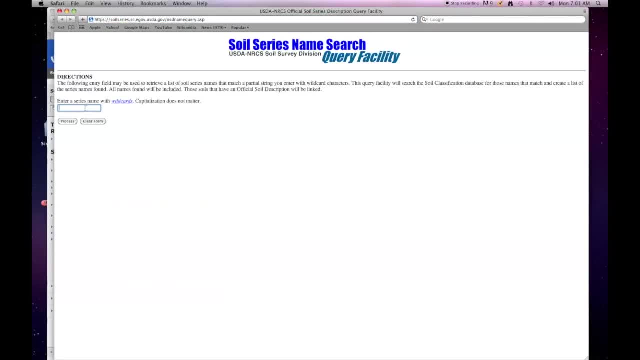 go to that search page and go and enter norfolk. okay, so there we go and i process that. and well, here it is. norfolk is a fine, loamy kaolinetic thermic, and i can view the description of that norfolk and it tells me all of the properties that you will. 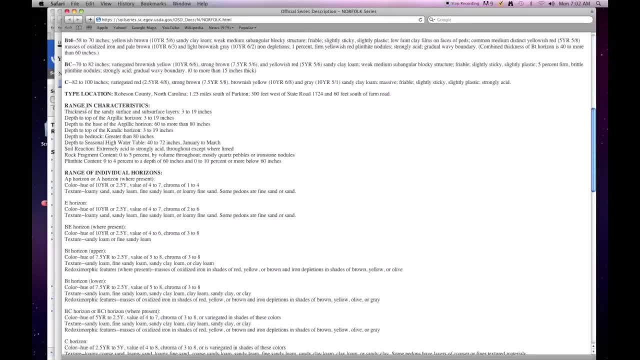 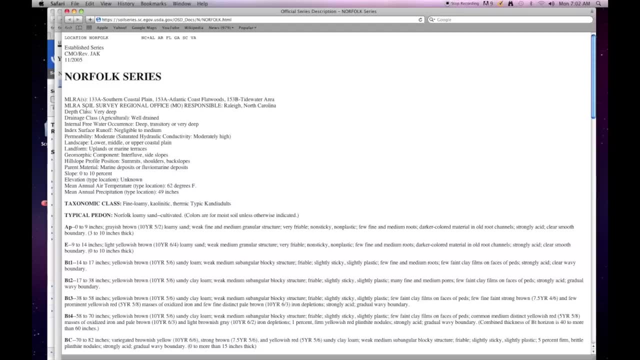 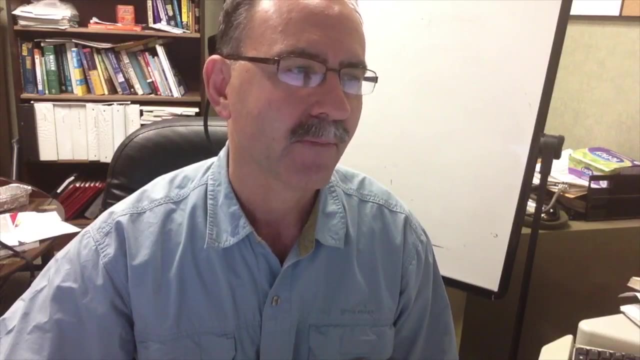 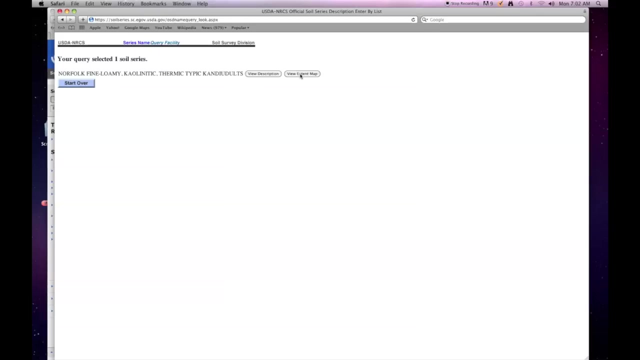 find in a norfolk cell, which is pretty, pretty impressive. these soil scientists- mainly guys who started out with the geologic background- were able to classify this information and it's been of tremendous use in this country. you can then also view the extent map, and if you view the extent map here, um, you will see that okay. 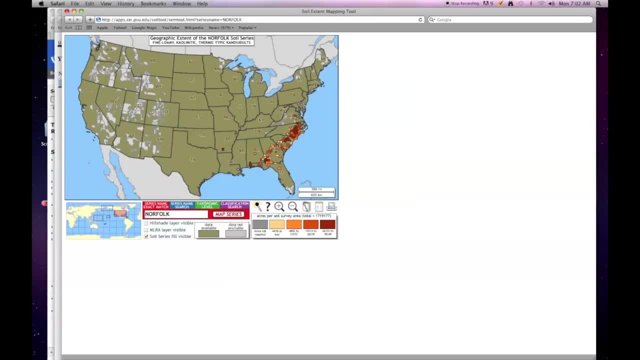 all right, so you can view. if you view the extent map here you can see that norfolk, basically, is, uh, found across the southeastern part of the united states, so that's kind of a good resource if ever we were interested in looking at the properties and extent of a particular soil. so much for the usda resources. 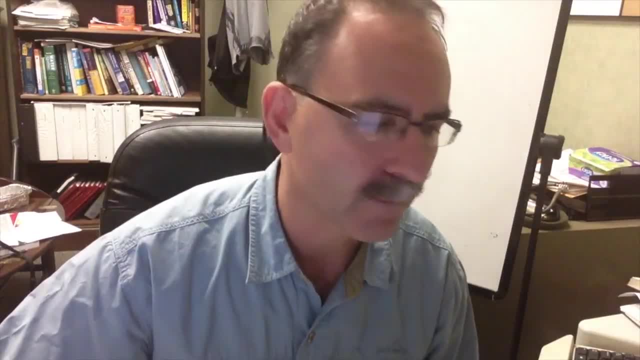 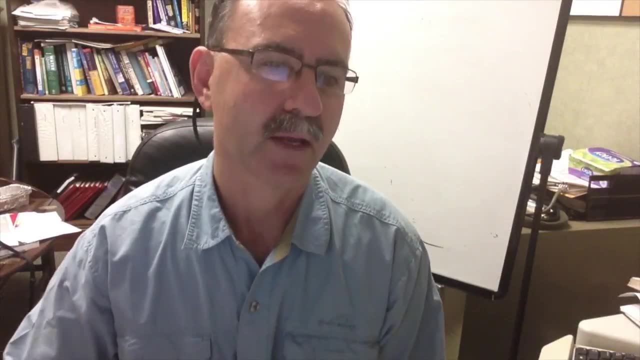 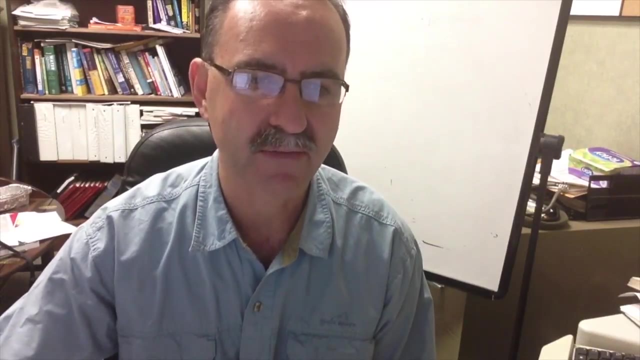 if you need to go there, you know where to go now. um, let's go back over here. so our alter, our um soil order, then is, uh, always that syllable in the last part of this very, very long name. so let's have a look at what soil order might seem important for us. soil order, then, is a. 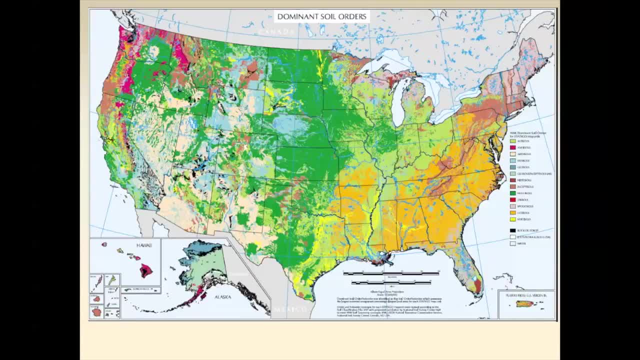 orders look like. If you look at the dominant soil orders in the United States you will see different. obviously these colors mean different things across the United States. In the eastern United States we have altisols. Alt usually means sort of advanced in process. These are soils that are weathered mainly because we have warmer. 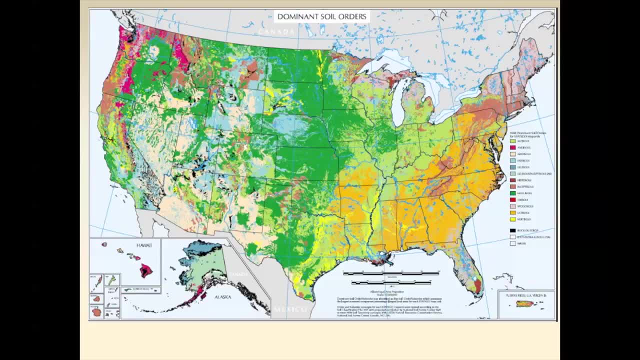 wetter climates, and so they're a lot more weathered than soils, say, in the Midwest. The mollisol is the soil that is most famous in the Corn Belt. It has a very, very thick topsoil, or what we call epipedon. It's a mollic epipedon. 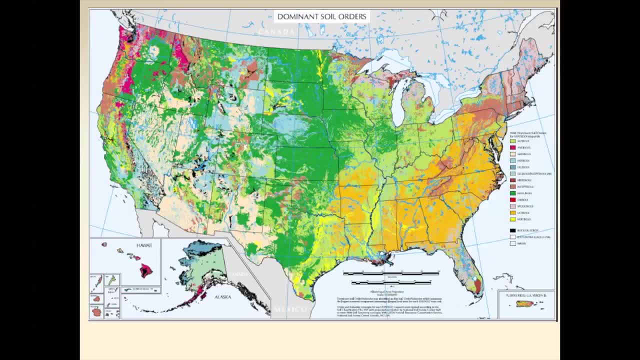 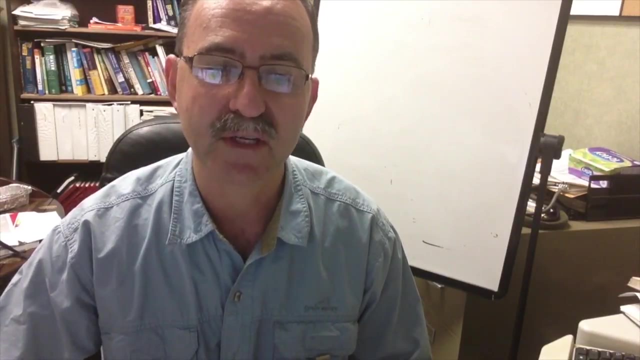 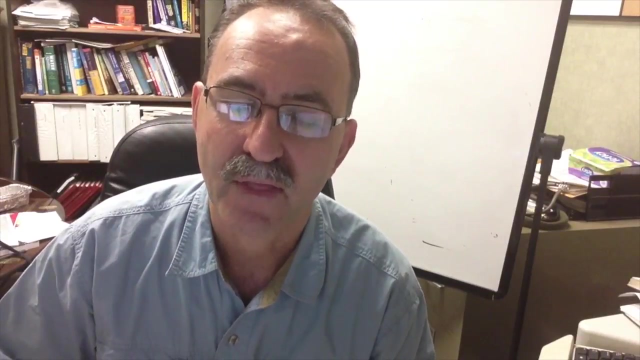 Moll is the word for soft. If you talk about mollifying somebody, you're kind of calming them down, And so mollisols are in this area. Other soils that you might find in South Carolina on the coast you'd find spodosols. You also find things called histosols. Histosols are soils that have very, very high amounts of organic matter in them- upwards of 20%. 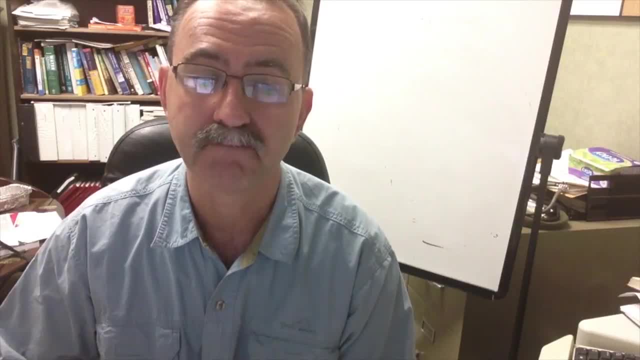 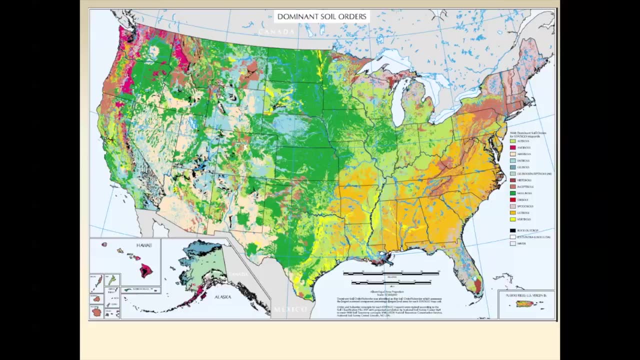 And we talked a little bit about Carolina. Carolina Bays would have that We also have in this part of the world inceptosols Inception means, or when we think about inception we think about early and there are some inceptosols, say in North Carolina, where you have the Blue Ridge Mountains coming out. 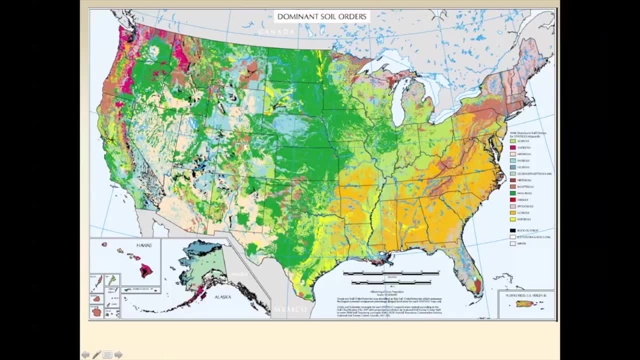 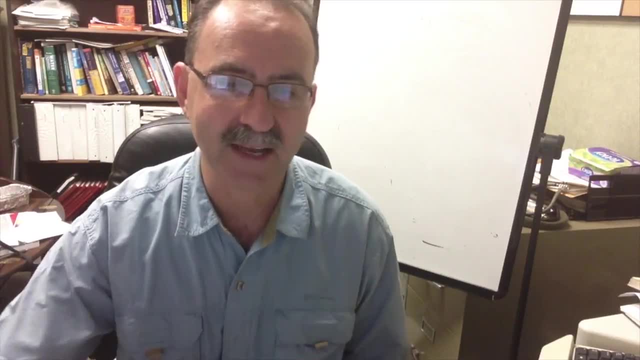 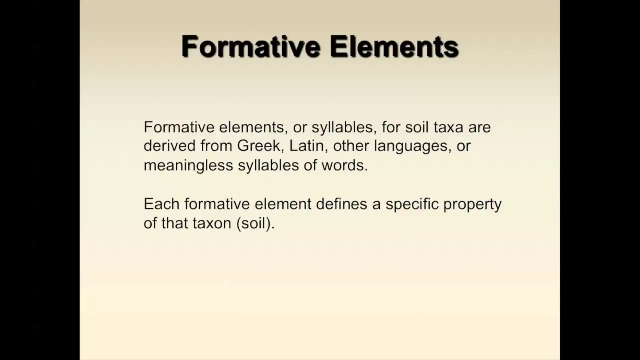 And there are a few more in this area Which we'll be able to find, of course. Okay, so let's leave it for that, because we can have a look at some of those names. The formative elements or those syllables for the soil taxon are usually derived from Greek, Latin or other languages, or sometimes they're actually meaningless. 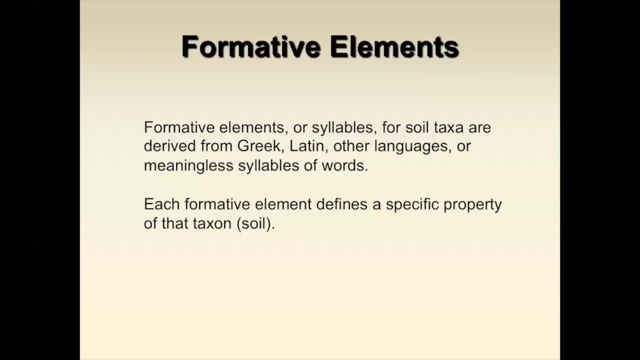 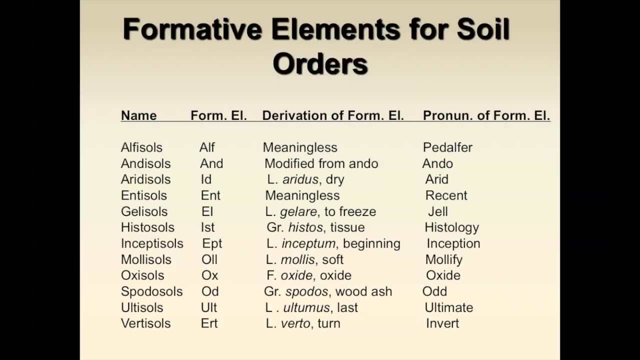 So each formative element really defines a specific part of that taxon. So, looking at the formative elements, The formative elements of those 12 soil orders- I'm not going to go through each one of them, but some of them make sense. some of them don't make at all any sense at all. 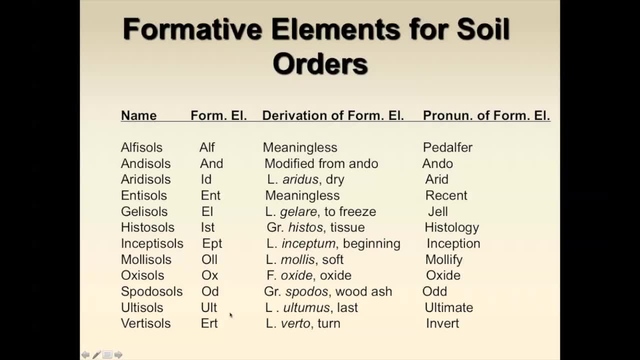 But, for instance, when we talk about altosols- the Latin is ultimus or last ultimate. we talked about it. it's well-developed. Oxosols, for instance, are soils that are found in tropical areas. 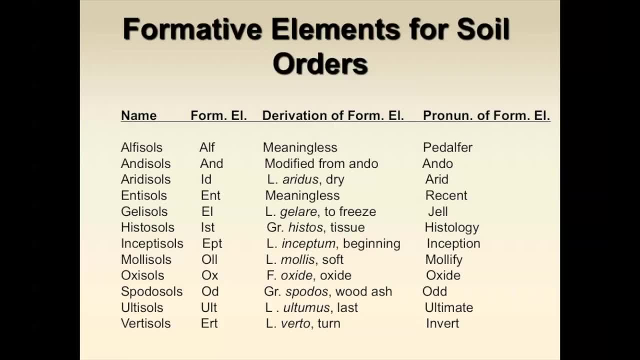 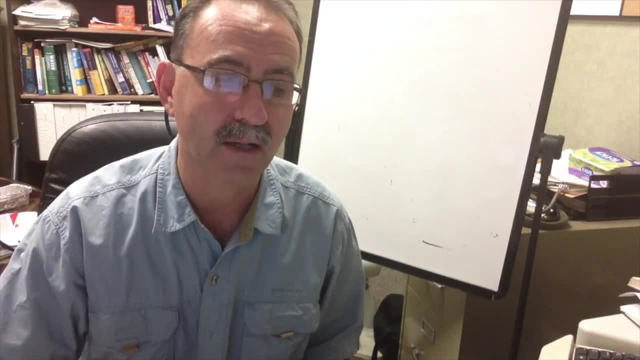 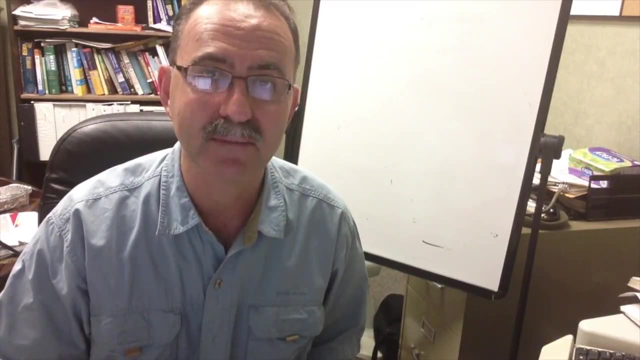 Oxosols, for instance, are soils that are found in tropical areas In Africa and Asia, where the soil has been weathered to an even greater extent than our altosols over here, So a lot of the calciums and magnesiums have been washed out and the soil is highly acidic. 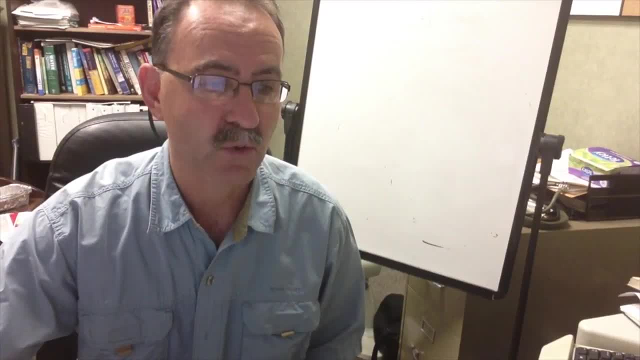 Molysools we've talked about. histosols we've talked about. So these are some of the soils that you're going to find. So these are some of the soils that you're going to find, and let's have a look at that. 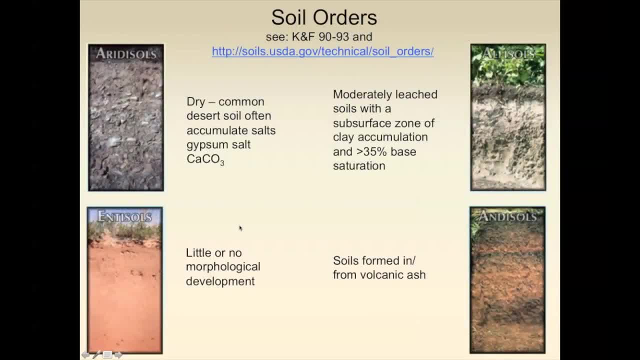 So these are some of the soils that you're going to find and let's have a look at that. have a look at each one of them very, very quickly. so, if we're looking at them alphabetically, if you want to actually go and get a map of these and pictures of them, you're welcome. it's going to be. 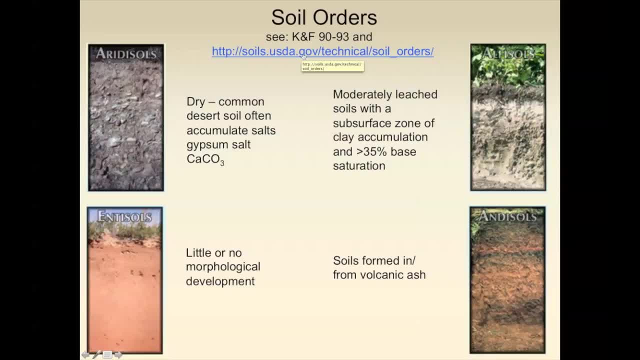 at the at this url over here. but aerosols are going to be dry and very, very much common in desert environments. going to be out in the west, okay, um, alpha salts over here are moderately leached soils with a subsurface zone of of clay accumulation and less than greater than 35 percent. 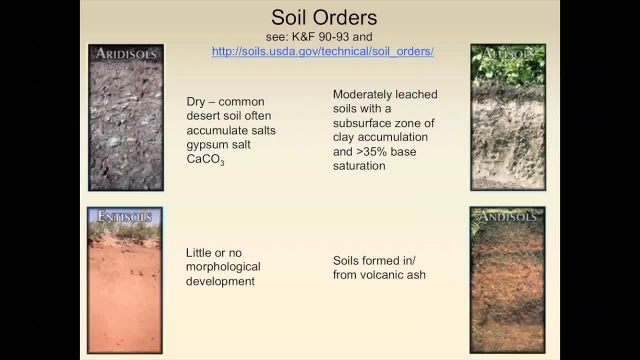 base saturation. base saturation is something that we'll look at later on, but it's related to the cation exchange capacity, and if you have greater than 35 percent of base saturation, the it means that you have, uh, greater than 35 percent of your cation exchange capacity sites. 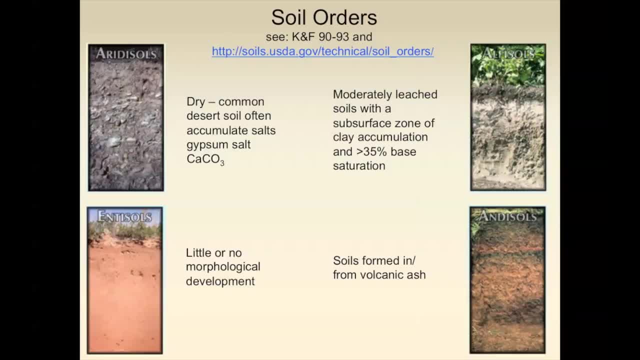 are occupied by calcium, magnesium or sodium ions. those would be some of your poor, your base ions. there's one other ion which escapes me right now: enter salts. um, you will see that there's very little morphological development on these enter salts and and you it's very difficult to distinguish from one soil horizon to the 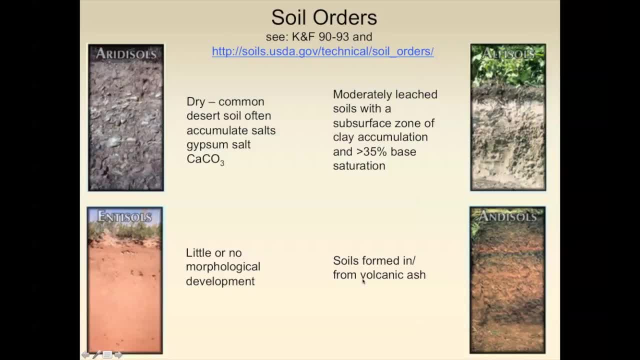 other, and the salts are soils that are specifically formed from volcanic ash. a place that you might find these is are, you know, art in the west, where you have places like mounts and helens, or possibly in hawaii, where you have a tremendous amount of volcanic ash. that's. 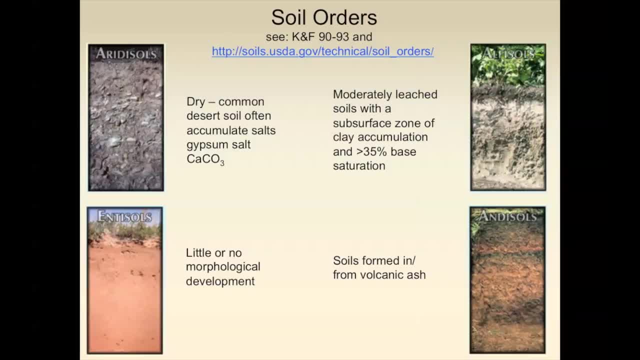 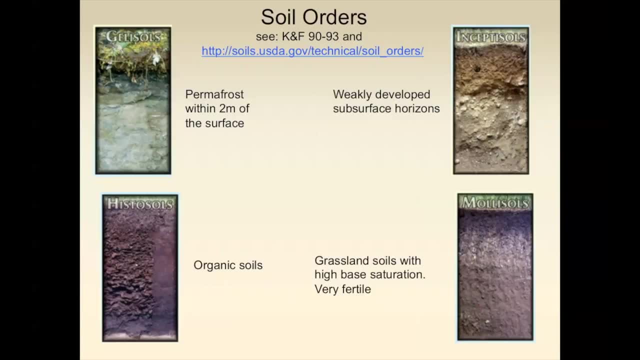 come out of. uh, that's history historically been there. uh, gel assaults are. when we think about, uh, gelati, the um italian word for ice cream. well, there it is: gel assaults. uh, in this case, you might have, you would have gel assaults where you have a permafrost within two meters of the surface. so these soils are cold and you would. 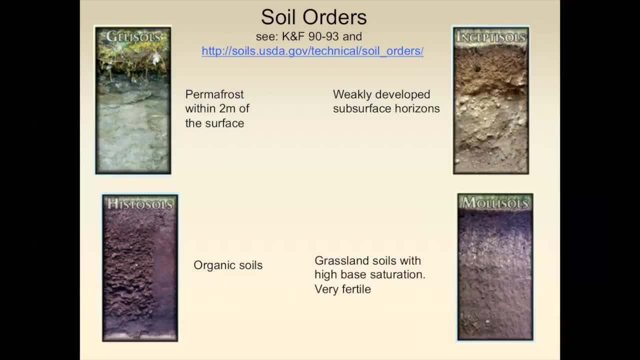 imagine that not much in terms of soil formation has happened in here, simply because so much of the time there's a lot of ice around and so you don't have that much in terms of shrink, swell or plant growth. your plant growth is mainly going to be things like: 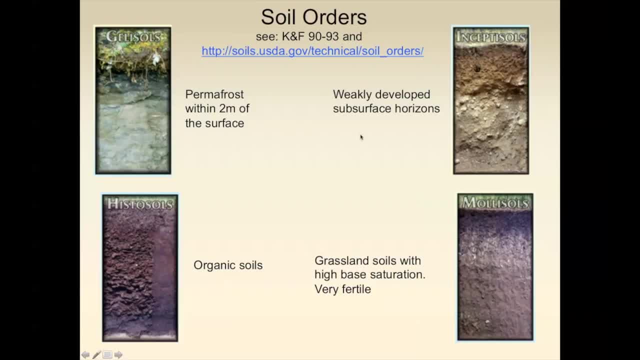 lichens or something like that. um inceptor salts will find some of these in the blue ridge. these are very weakly developed sub surface horizons, relatively speaking from a geological perspective. they are going to be young soils, and so they will keep going on like we've done over the next couple of years. 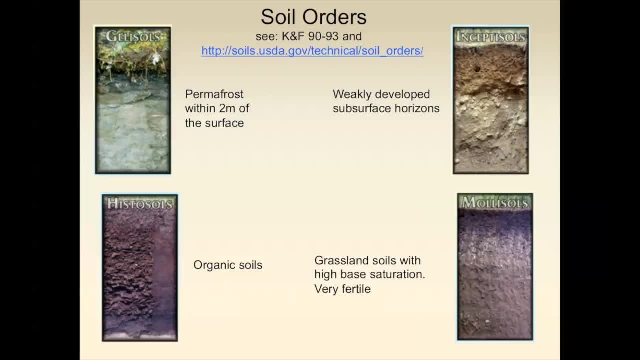 at the inception of their formation. histosols: I talked about these as well. they're organic soils and we would find them in Carolina bays in in South Carolina and North Carolina, for that matter. the mollusks are these grassland soils. remember- I think it was last week when we talked about grasslands where you had these grass roots that grew down maybe five, ten foot into the, into the A horizon and sometimes into the B horizon, the subsoil. and when the grasses die in the winter, the roots often would die as well and become organic matter, and so these mollusks. 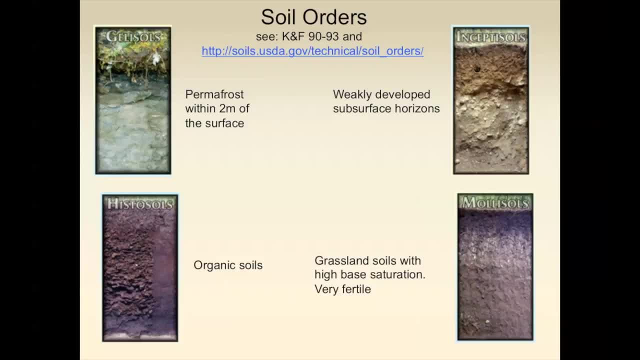 soils are the grassland soils- very, very high base saturation, very, very high cation exchange capacity. that means that they can- oh sorry, they can- they can hold lots of cations, cations potassium, above bacillus saline or intrusive water. so it's a very high-quality base saturation可愛, very, very. 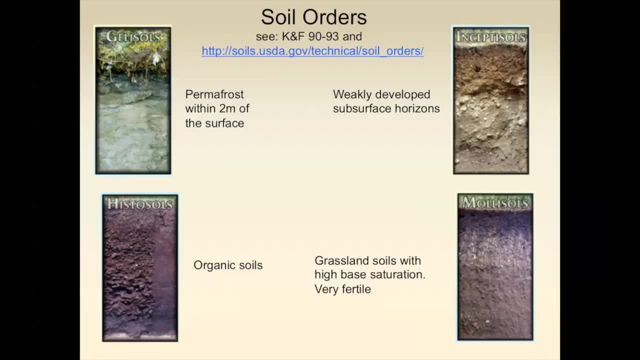 or anything you create, called a mull, Even the eaten and the on top next slide out. you have. you are, of course is the most important- Potassium, calcium, magnesium and sodium. Extremely fertile and you'll find the molluscs if you go back into that soil order map. the 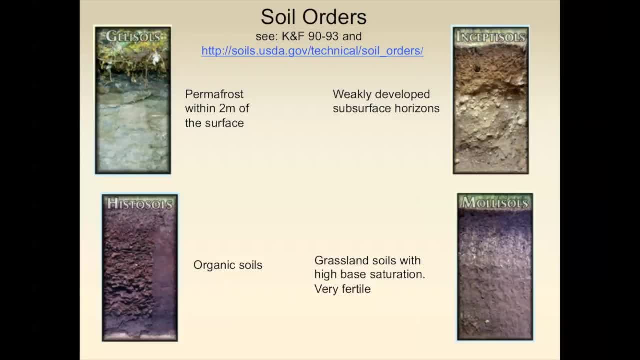 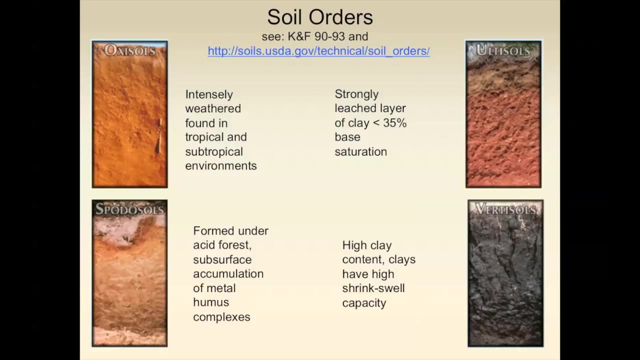 molluscs are going to be in your corn belt. That's where they grow the most corn, Very fertile and holds a huge amount of water as well, because they have these deep A horizons. The oxys salts are intensely weathered soils found in tropical and subtropical places. 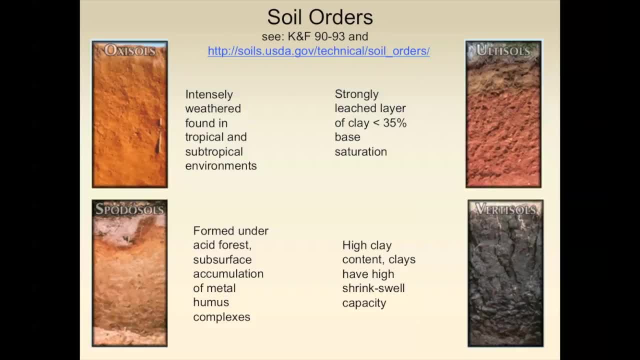 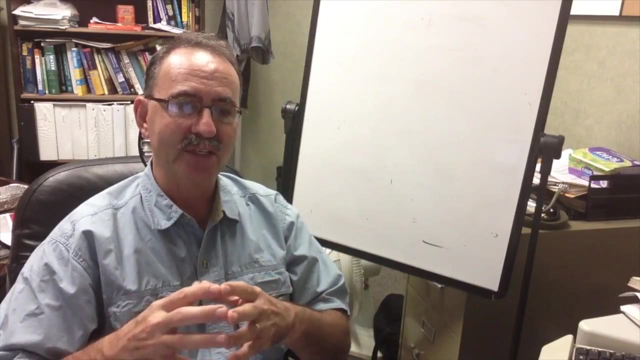 I mentioned Africa and Asia, but South America as well. So, for instance, a lot of the soybeans you find that are grown in the Amazon basin, for instance, are on oxys salts, So they've got to deal with some of these fertility issues. Very intensely weathered Alta salts are also. 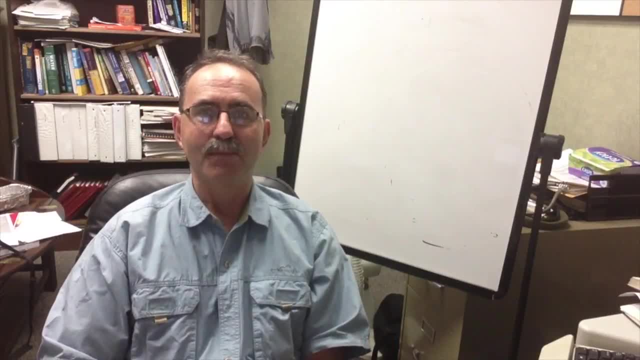 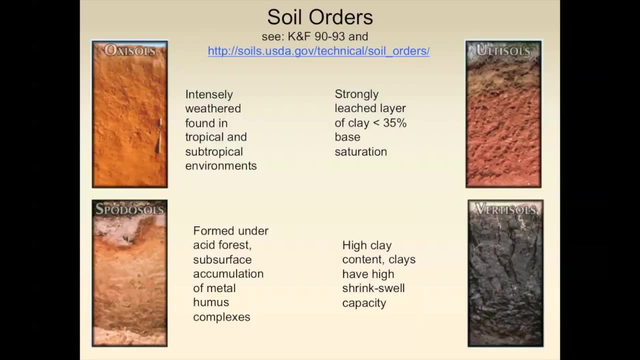 intensely weathered, So it's not as bad as oxys salts. but as a result of very warm, very wet weather, In this case the clothes have less than 35% of base saturation. In other words, less than 35% of your cation exchange capacity is taken up by some of these- excuse me- cations. So 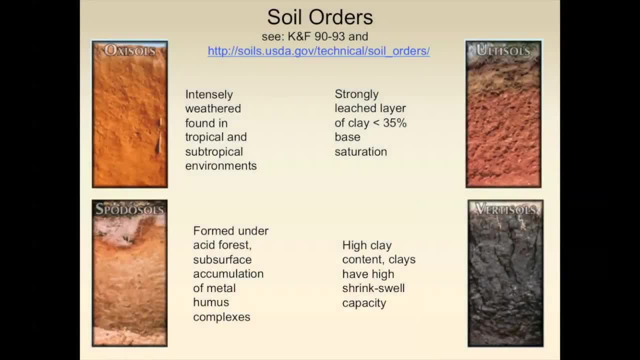 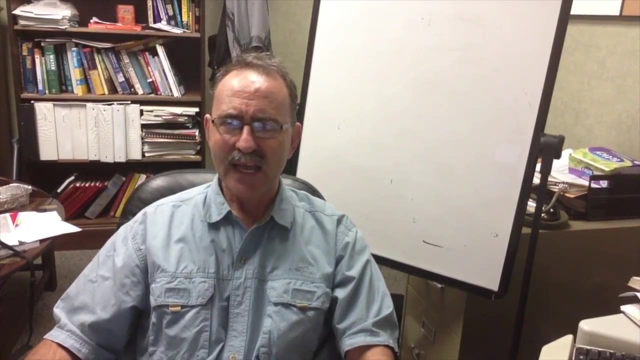 it's not completely by by these, by these cations- potassium, magnesium, calcium, sodium, Spodosols are kind of odd soils And they're formed usually under acidic forests and in sandy dune, swale kinds of areas. You'll find find Spodosols down in Charleston And what happens is that you you have a very thin A horizons. 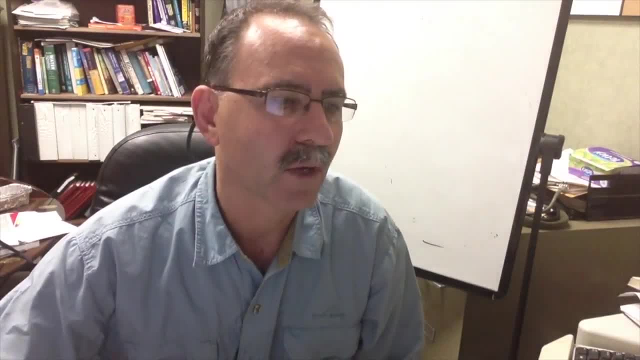 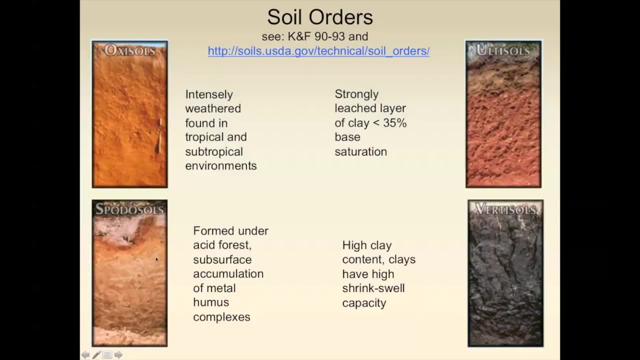 But when you go down to your fron, you, you can see that horizon, and then you'll find that a lot of your metals, your irons, your, your minerals have leached down into your, your B horizon, and sometimes even you see horizon and often this might be, you know, you might have a. 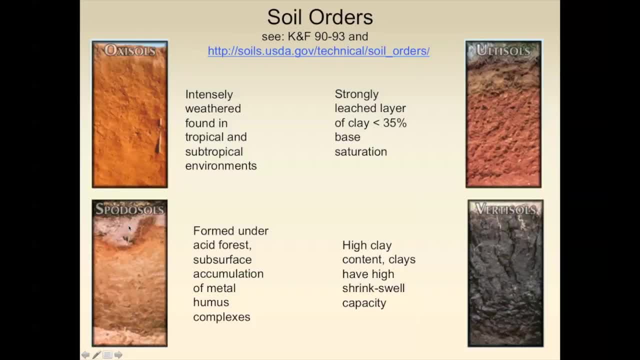 very strong deep horizon and then after a while- maybe a two or three foot- you'll find this strong layer over here of where your clays and your minerals have accumulated. and then your vertisols are soils that have very high clay content and you can see they have extremely high shrink swell capacity. so the clay 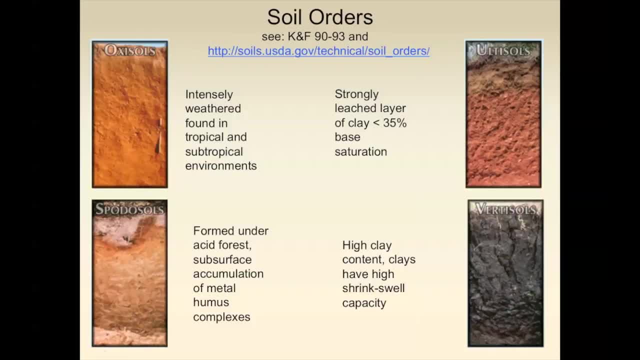 contents in this case are not clays like we would find in the southeast. in the southeast we have kaolinitic clays which don't shrink and swell much. these clays are shrink and swell a lot. it might be those names escaped me right now, but we're 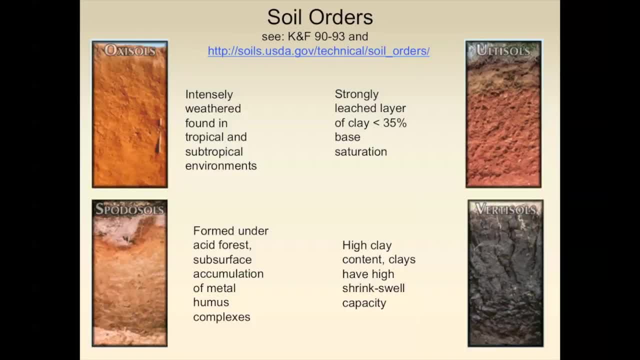 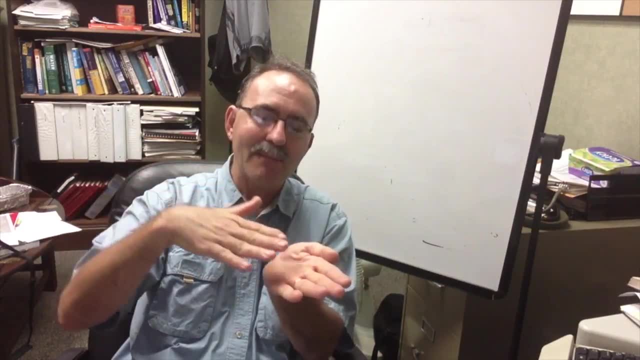 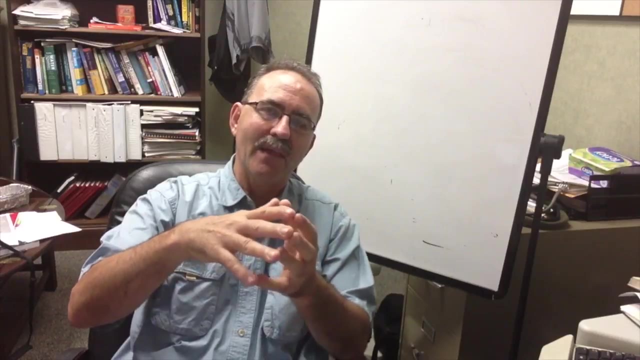 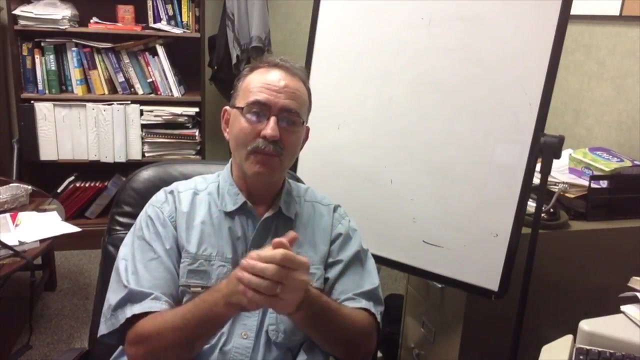 going to talk about that in some clay mineralogy later on. but these clays are layered in such a way that water and minerals can actually come in between those layers. and when water comes in between those layers it actually expands it, so that clay then spans and when it shrinks, or when it dries, it's going to shrink and form these incredible cracks. 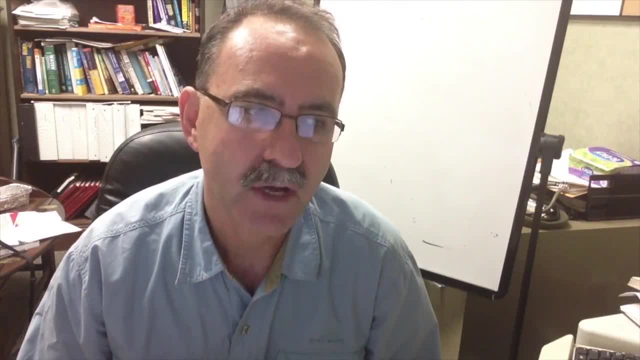 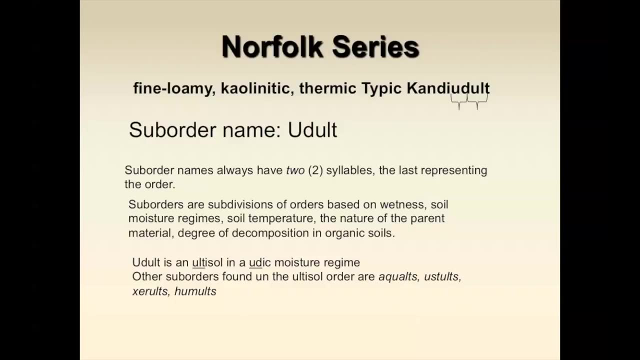 so those are. those would be vertisols. so much for the soil orders. um. you then start to look at um. going back to the norfolk series, the norfolk, if you just look at the sub order name, is: remember, the order name was alt. the sub order name is now going to be: it's a udelt. okay, so you ud. 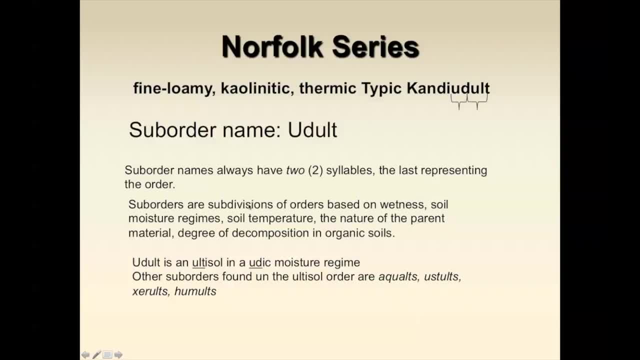 refers to the fact that it is a eudic soil. it it's the wetness of the soils, so some orders are subdivisions of orders that are based on wetness, soil order regimes, soil temperatures, the nature of the parent material, possibly, or the degree of organic decomposition in in those organic soils. 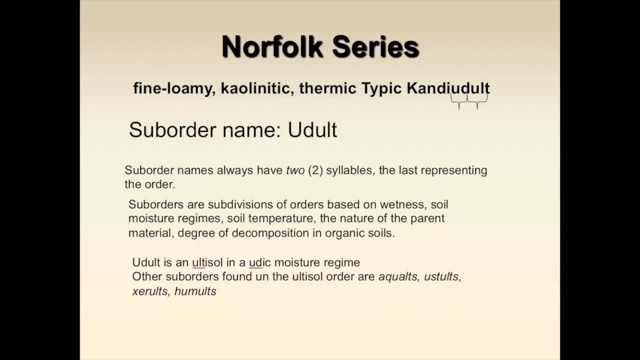 so the udelt is an altosol in the eudic moisture regime, so let's go have a look at that map and see what it looks like. other sub orders found in the altosol area are going to be aquilts. so aquilts, you can imagine, are aquic soils, soils. 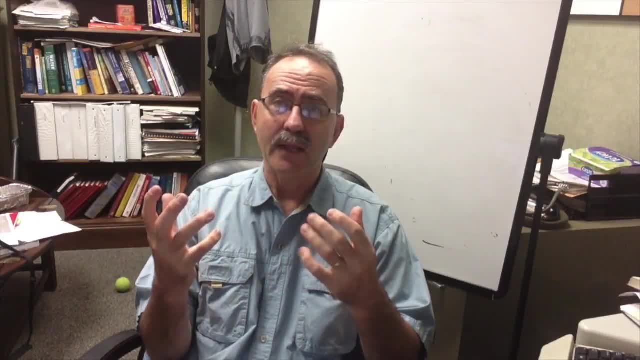 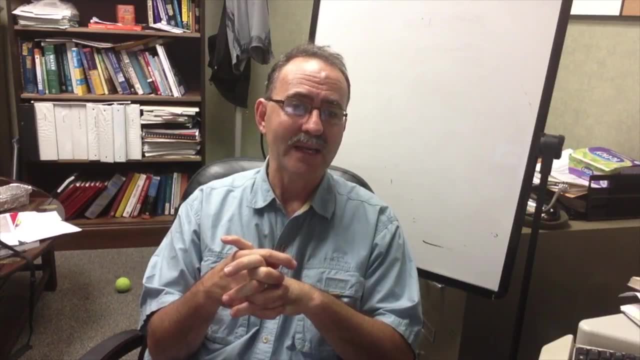 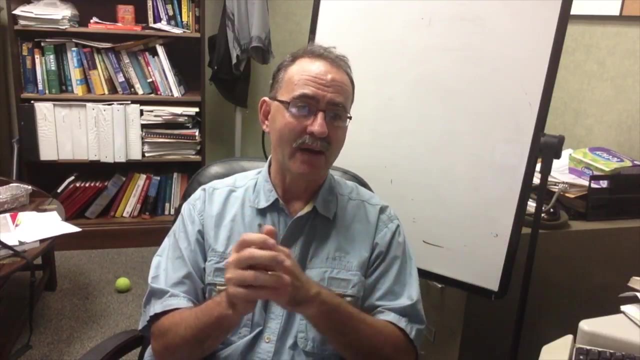 that are very wet in in the altosol range: eustelts, which are going to be soils that are not quite as wet as udelts, xeralts, which would be soils that are altosols but in xeric environments and humults, humic would also, I think. 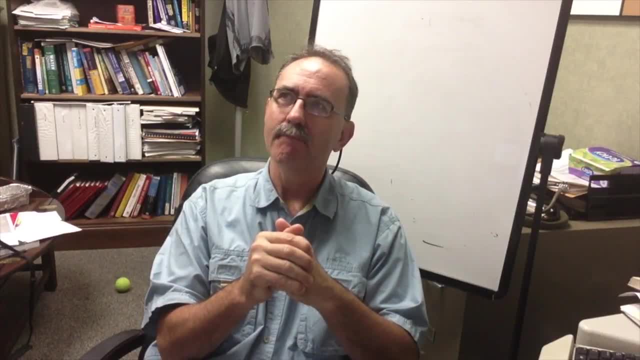 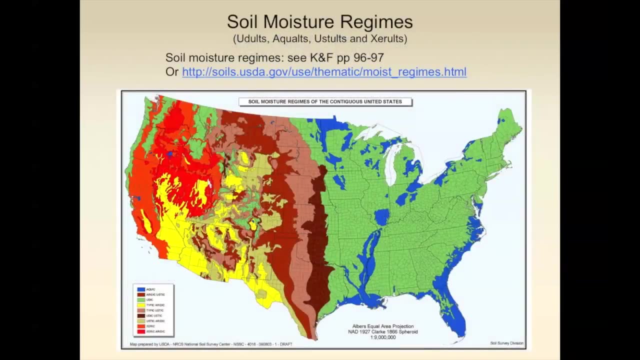 really it's not histic, but it would have a lot of humus. I think I'm you, I'm guessing now on that one. but soil moisture regimes that we can look at. you can see the eudic moisture regime, so that green part is going to be across. 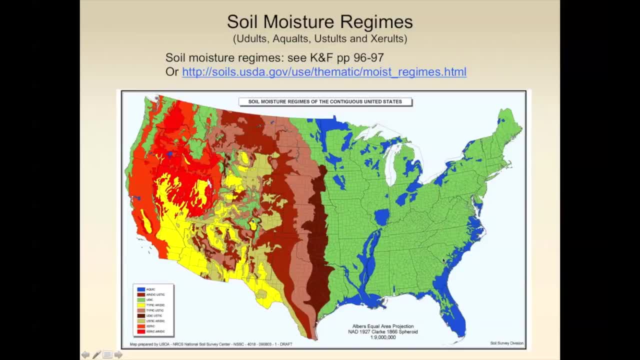 the most, mostly the eastern part of the United States, the aquic moisture regime going to be down the Mississippi Delta area, up in the Minnesota lake regions and then of course down in the southeastern seaboard as well, these coastal plains. so those are some of the major soil moisture regimes in this. 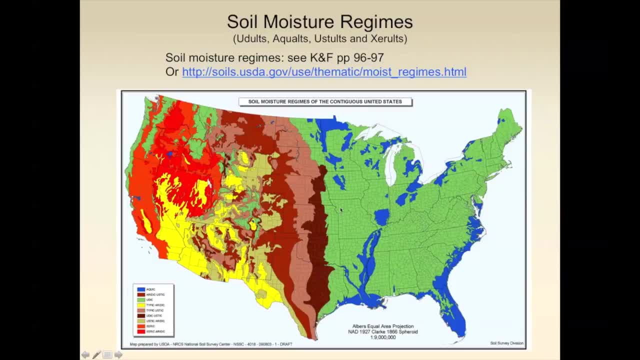 country. what you now begin to go over here is the eustich. we talked about those moisture regimes, I think, in the second week, and then we get into the xeric and eridic soils over here. remember the xeric is going to be a mainly the mediterranean kind of climate where you have cool wet winters. 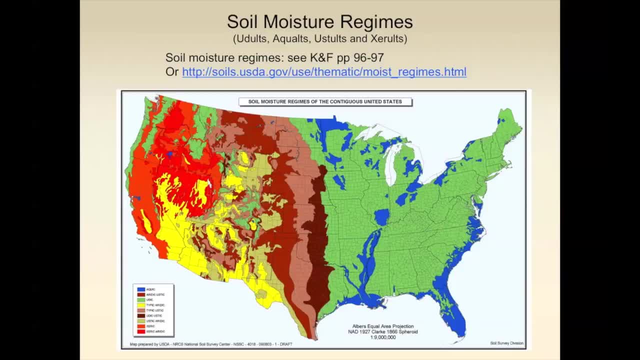 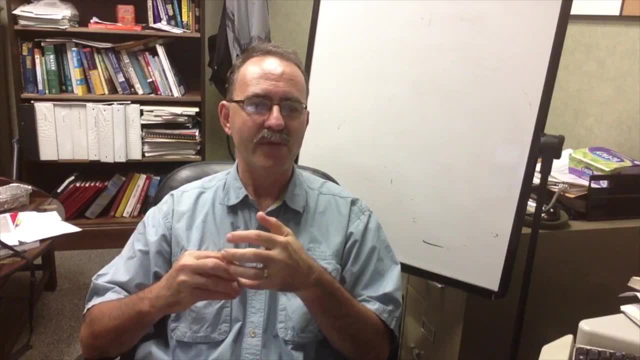 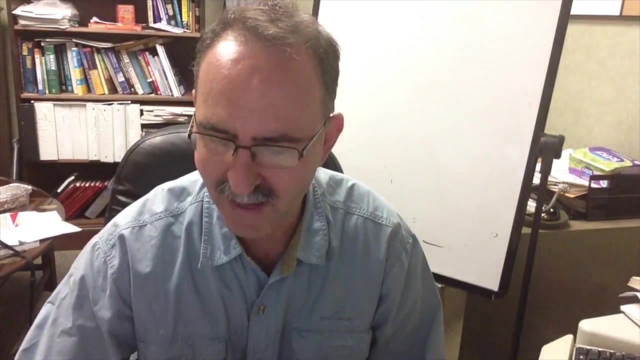 and warm, dry summers. and then of course the eridic is going to be places like Arizona where you have year-round you have very little rain at all. so that kind of gives you that soil moisture regime. look again, you can go to your maps for that. so other soil sub-oil: 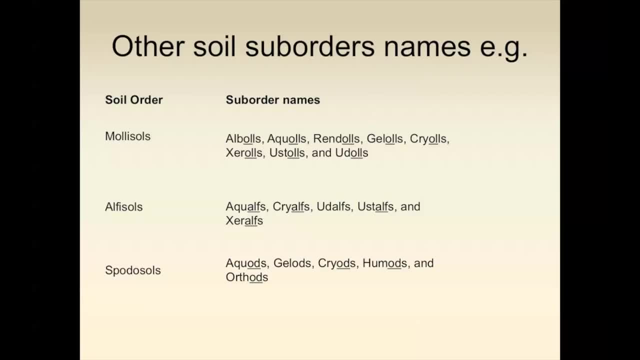 order names might be. for instance, if you have a monosol out in the west, you may have an albol albic, I think. if you think about an albino, albic would be a fairly light colored soil. aquil would be a monosol that has an aquic. component: very wet soil. gelol, for instance, would be a monosol. that that is, gels and cryols would be monosols that are extremely cool. the same thing with some of these other soil orders that you see. so you can derive. take a look at these and see if you can derive from what. 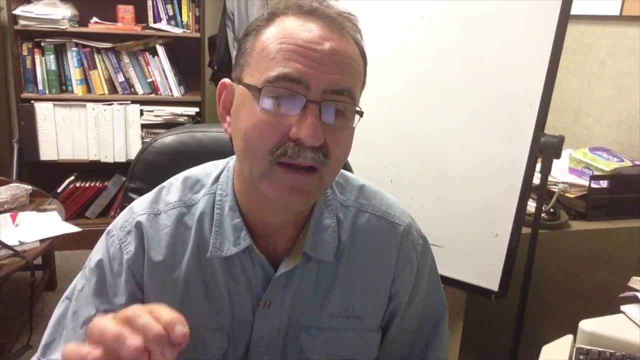 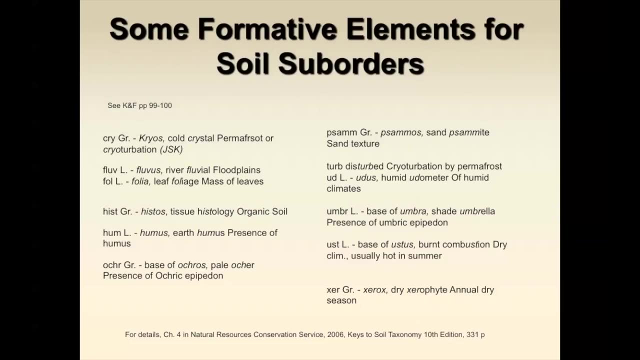 they're saying from these sub-order names what kind of soil properties you might infer from them. so some formative elements of those soil sub-orders. again, you can go to Conker and Fransmeier and you can have a look at some of these four formative. 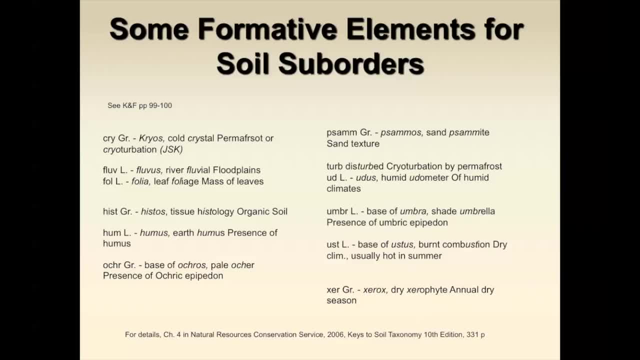 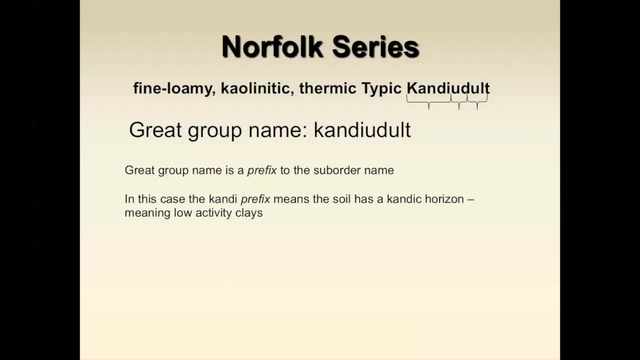 elements over here. I think Conker and Fransmeier does a good job of talking about soil taxonomy as well. in fact that's where I really was able to understand soil taxonomy a little bit better. so now we're looking at the great group name for the Norfolk series. so the great 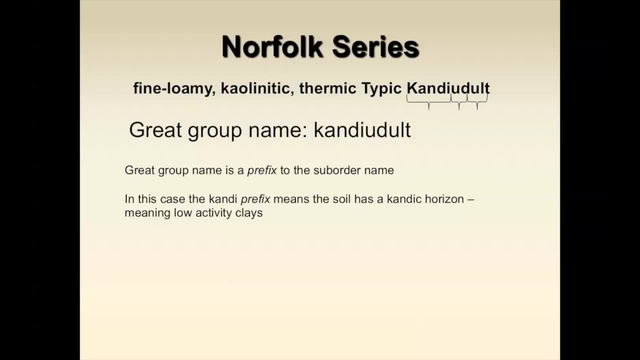 group name for the Norfolk series would be candy. you dealt ok, that means the great group. now, the great group name is a prefix for the sub-order name, so actually, let me so the great group name in fact would be this candy over here. so what does that mean? in this case, candy is a prefix for a low, for a soil. 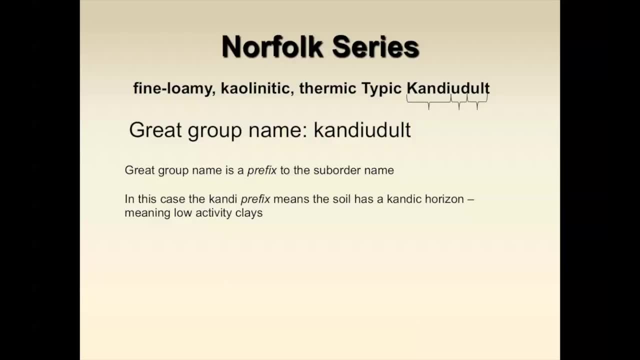 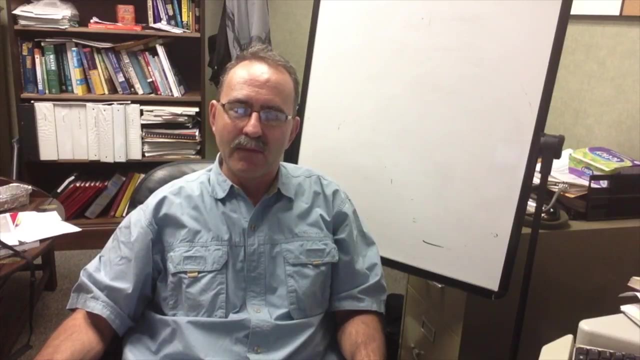 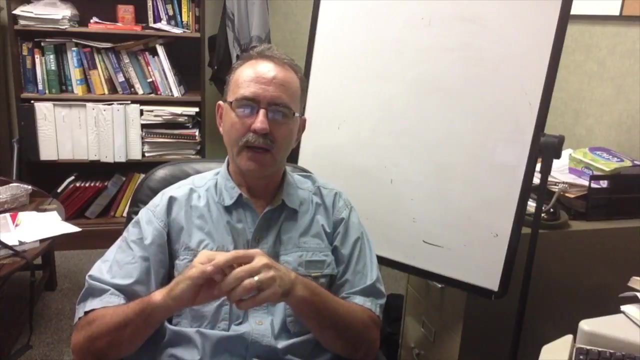 that has a candy horizon, meaning low activity clays. we have low activity clays in this part of the world. they're one-to-one clays. they're kaolinitic, they they don't really shrink or swell and they're fairly tight and so they don't really allow that much in the way of cat irons to come in between. 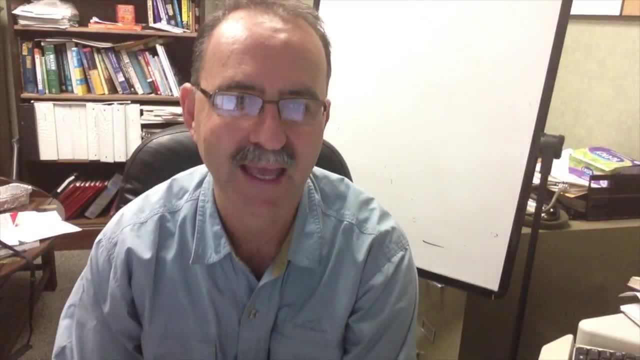 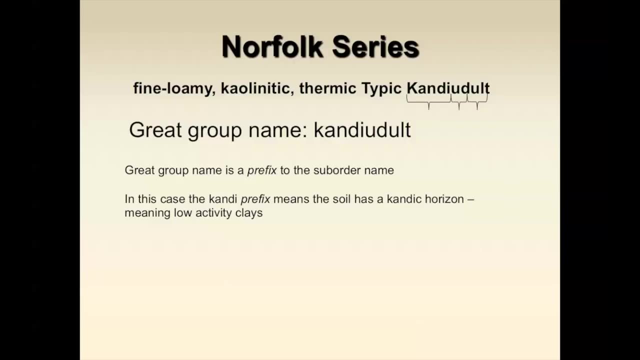 each of those layers. so that's what we mean by a candy, a candy soil. so Norfolk series would be a candy you dealt. so, each going back here, each one of those, this syllable, this syllable and then this, if you, if you like these two syllables, carry with them very specific. 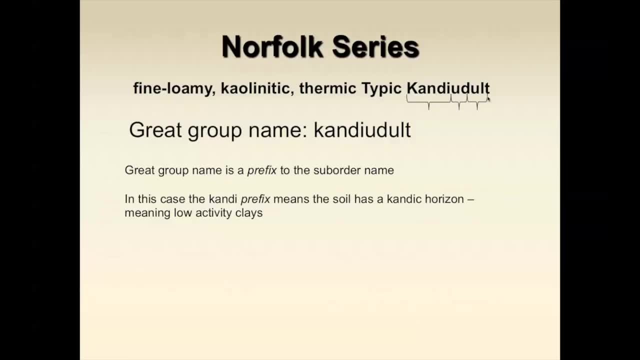 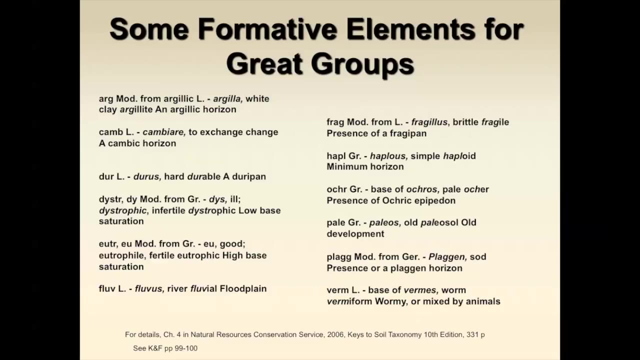 meanings. ok, um, some formative elements for great groups. now i'll let me just go back and formative. Elliot said these are descriptions now of the sub orders, or prefixes are general, would be a white clay, so you might have an argillic horizon, a cambic horizon, a duris. 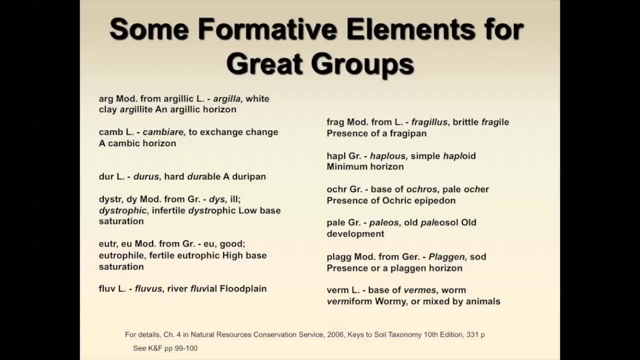 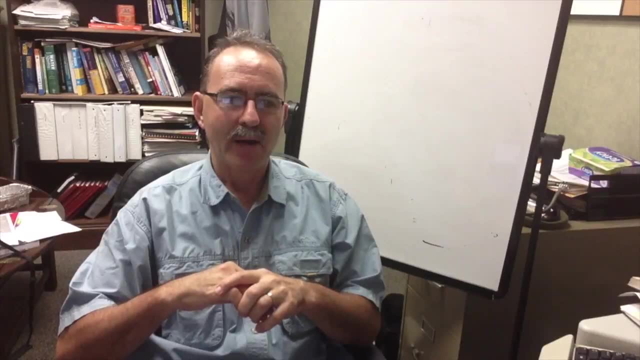 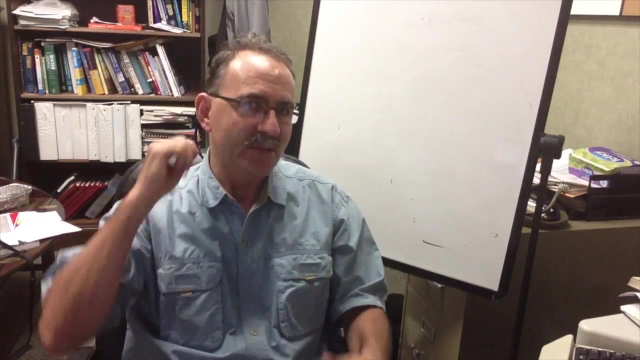 or a durable horizon, a duripan which might be a hard pan. hapless horizon would be minimum or not very well formed. ochric often meaning pale, pale or paleos meaning old. So again you can see some of these formative elements and again these become part of your. 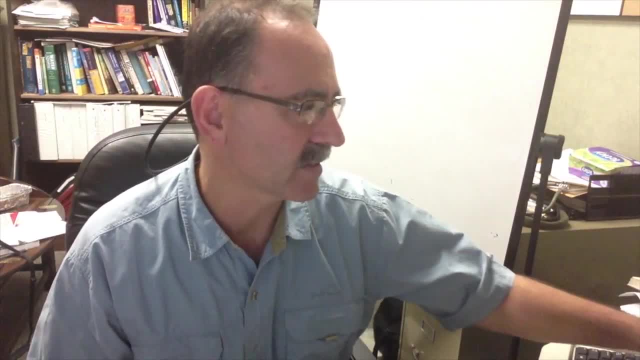 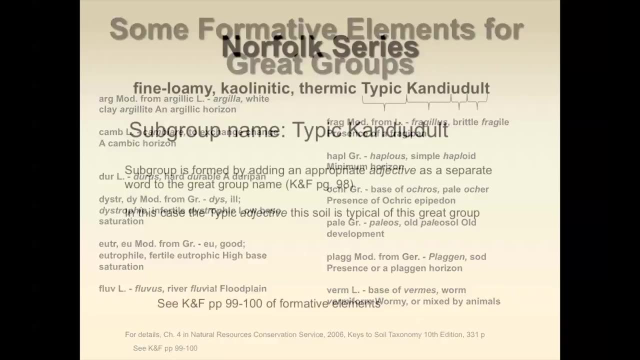 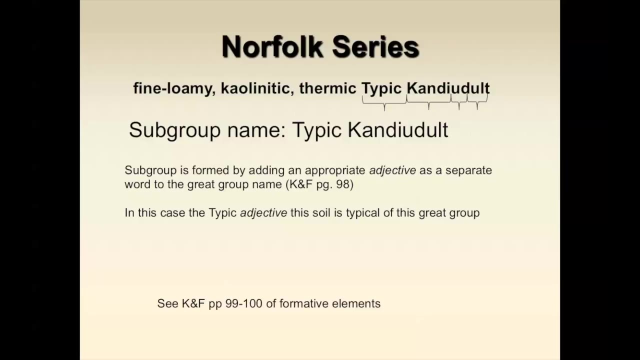 phrasebook in being able to classify soils and again go to Conker and Franz Meyer to make sure that you have that phrasebook down. So now we look at the subgroup name. the Norfolk series is a typic candiudal. the subgroup: 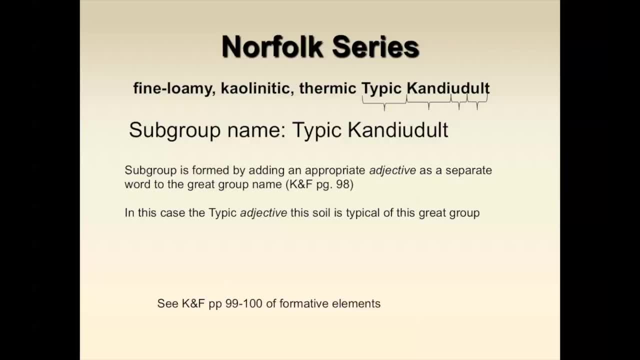 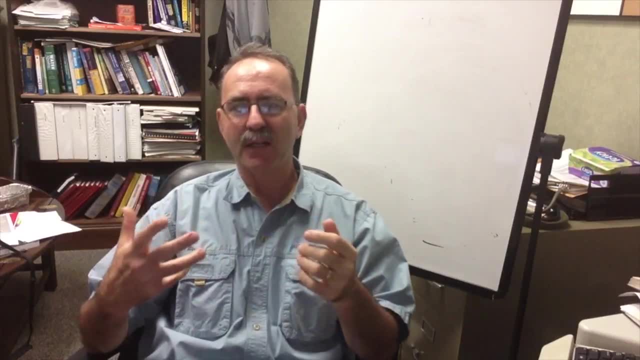 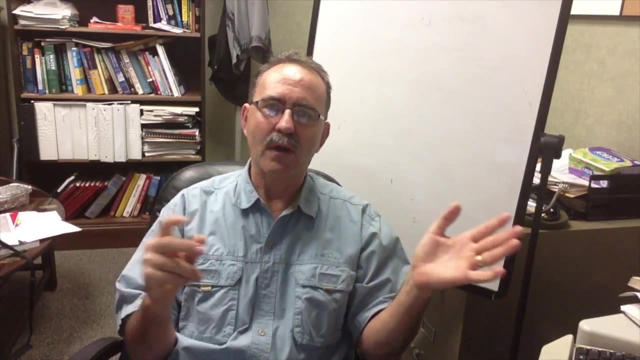 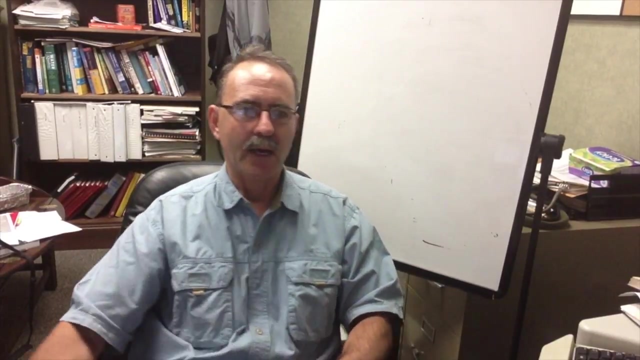 name is found by adding an appropriate adjective. so typic would mean, in this case, a typic adjective is. this would be typical for this great group, you know. and so if you look at a whole lot of candiudals, the Norfolk series would be typical of many of those candiudals. 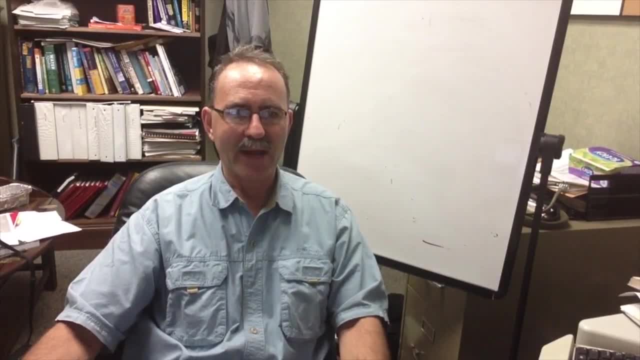 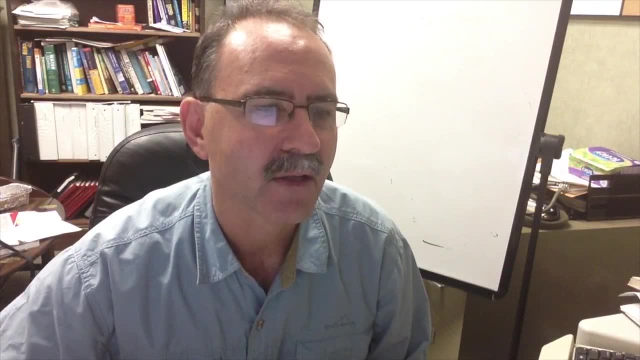 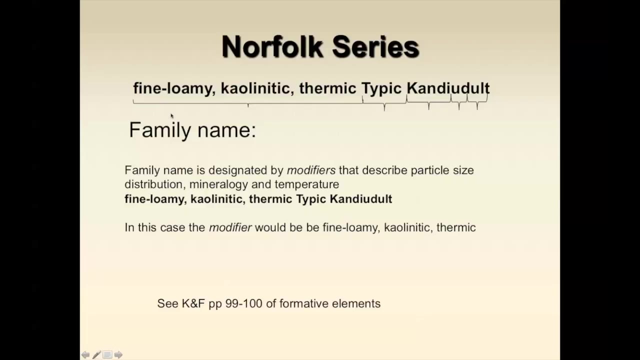 Now you're starting to look at the family name. over here we're at the sixth, so it's one, two, three, four, five. this is your family name. it's designated by modifiers that describe particle size, distribution, minerality, temperature and also how this. 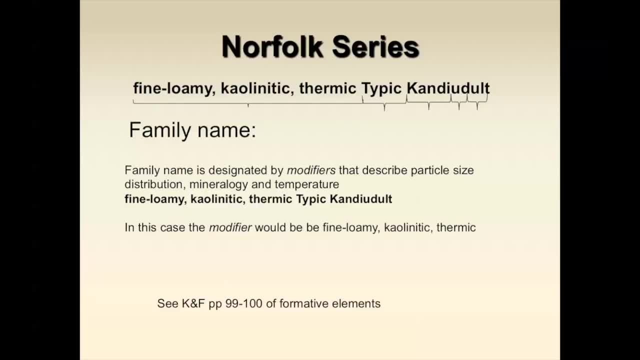 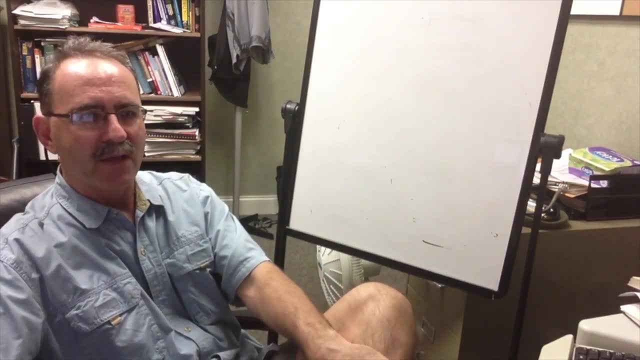 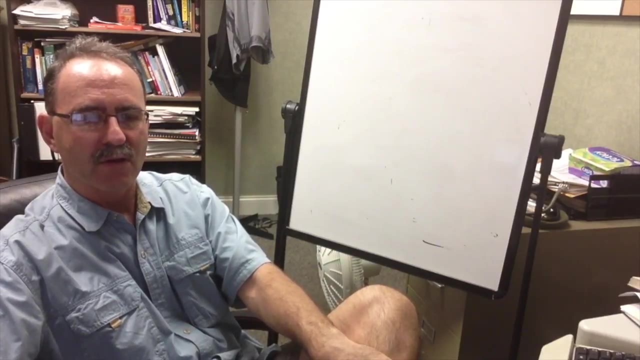 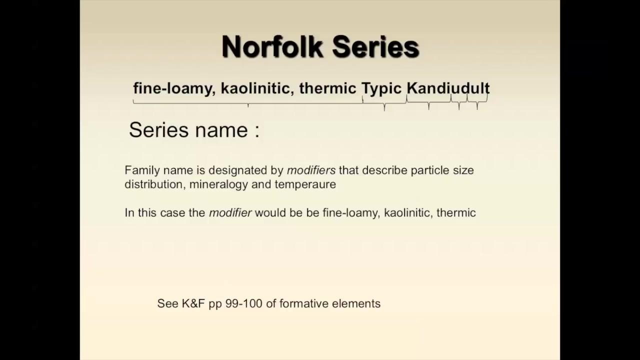 soil may respond to management. so in this case our family name or the modifier over here is going to be Your fine loamy kaolinitic thermic modifier of this typic candiudal. I hope this makes sense over here. 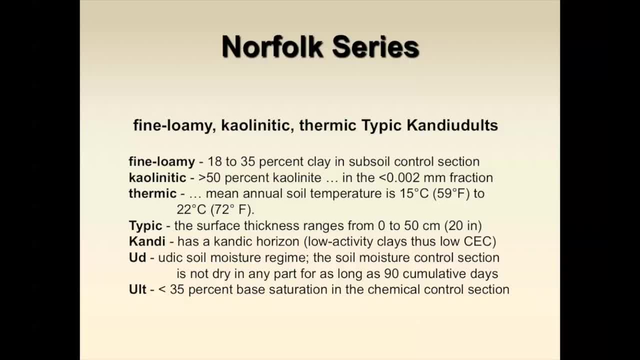 So your Norfolk series is fine: loamy, kaolinitic, thermic, typic candiudals. so let's go back again. The alde over here is less than 35% base saturation. that's probably one of its main qualities. 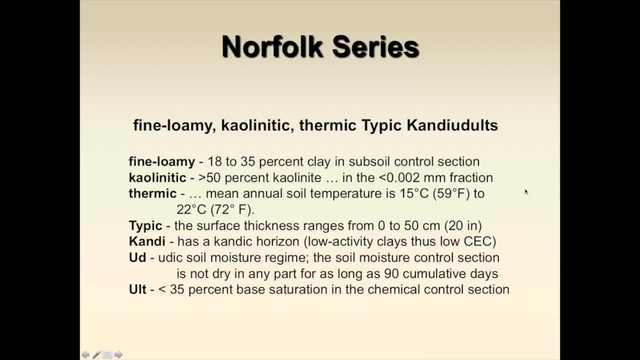 of these alde soils that you'll find in the southeast very, very well, excuse me, very, very well- weathered soils, developed soils, The oud- over here it's oudic soil moisture regime. The soil moisture control section is not dry, it's basically a wet soil and there your 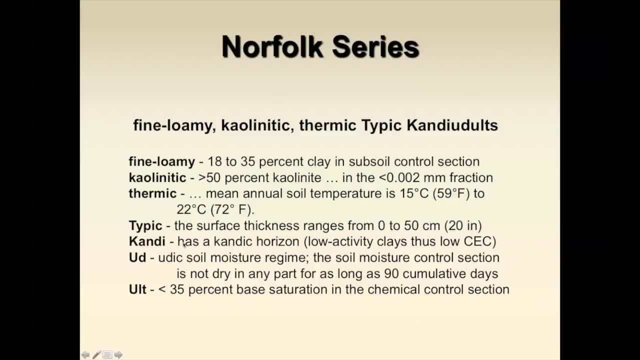 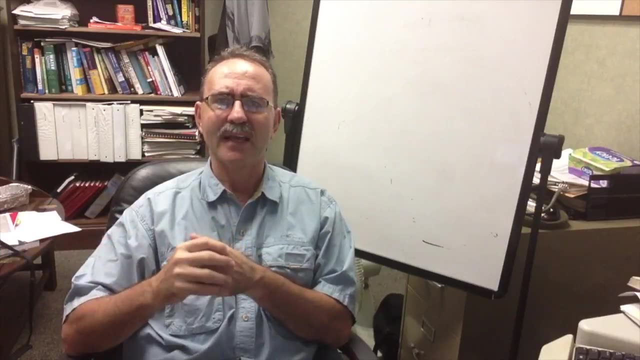 qualification of that is: It has a candic horizon. it has a very, very low. the clays in the subsoil are going to be low activity. that means they don't react as well as some of the clays that you'll find. 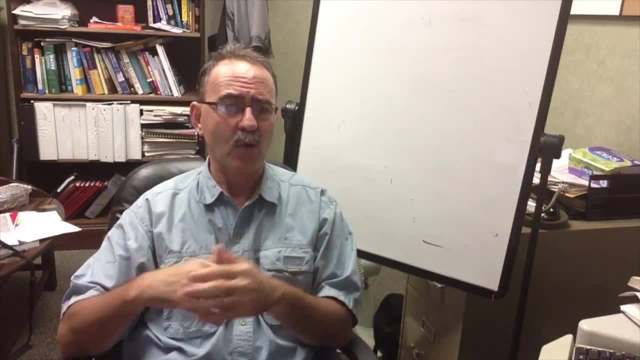 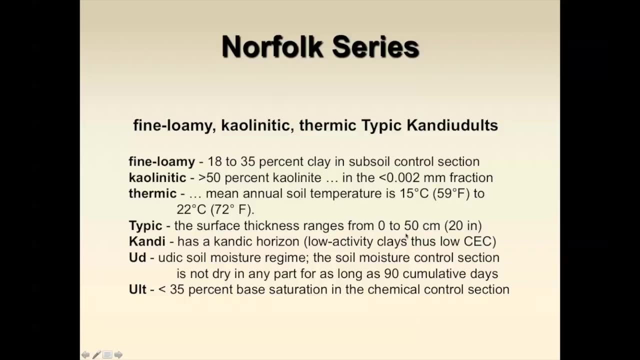 up in the northern part of the country in the corn belt. That's a good point. That's a good point, Thank you. Thanks so much. It's typical, and in this case the surface thickness ranges from zero to 50 centimeters. 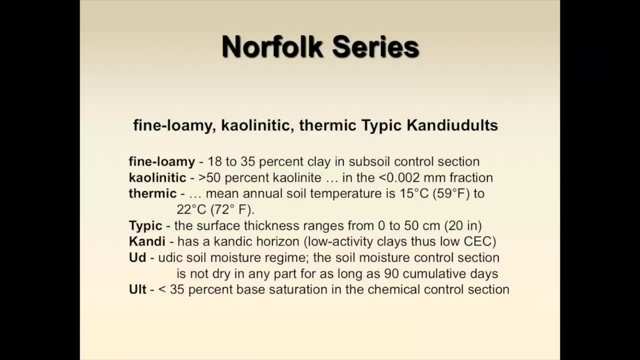 or 20 inches, So that's typical for what you would find in a candiudal in this part of the world. It's thermic, meaning that the annual soil temperature is 15 degrees C to 22 degrees C. It's kaolinitic, because it's greater than 50% of the soil moisture. 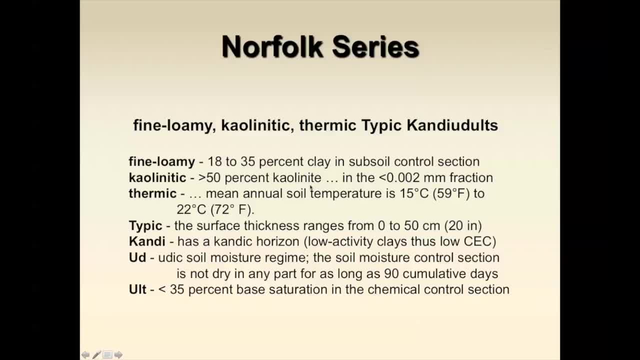 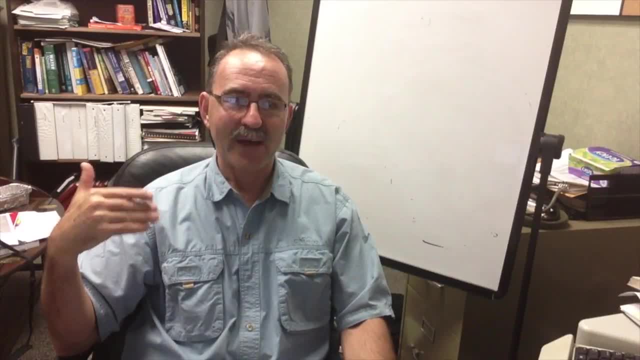 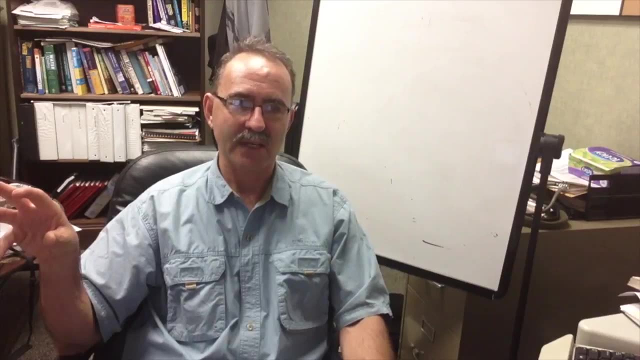 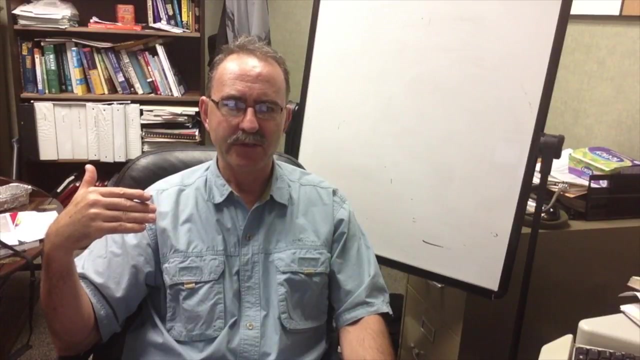 50% kaolinite- that is a specific mineral that we talked about, that low activity clay, and then finally it is a fine loamy soil. that means about 18 to 35 percent of this is clay in that subsoil control section. um, again, i'm not expecting you to be able to sort of learn all of these things. 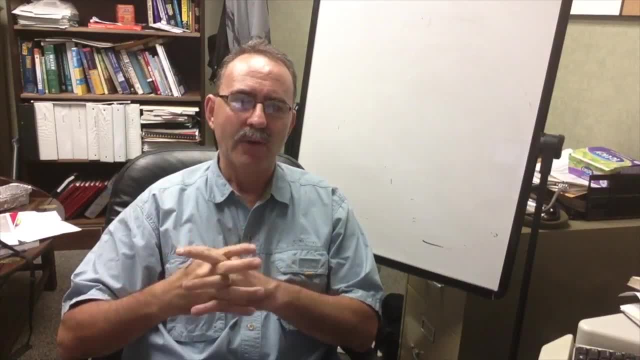 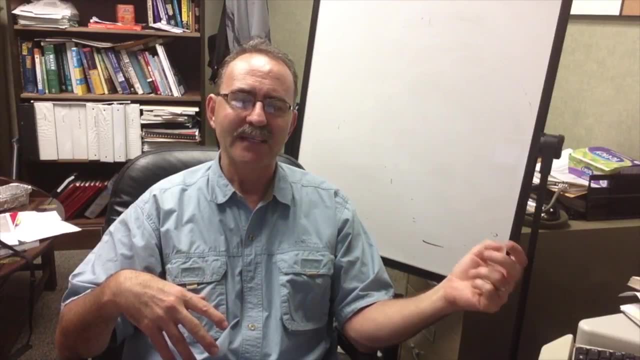 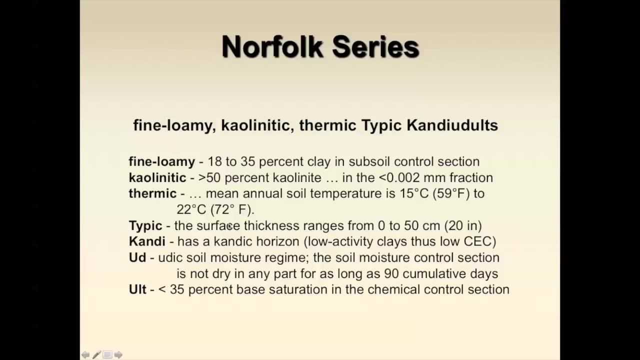 off by heart, but if you were in an exam, i would either give you all those phrases that you needed to. basically, if i gave you a soil description that looked like this, i would expect you then to be able, from that soil description, to be able to build up this name. remember your series name. 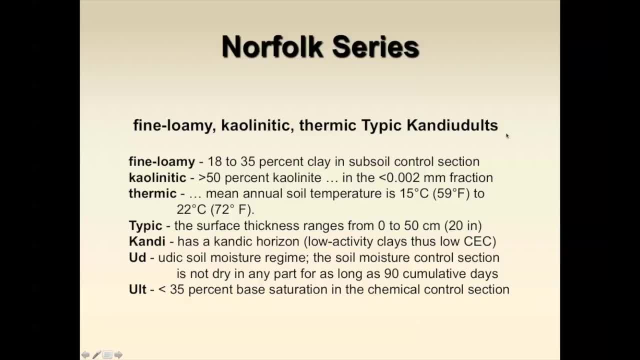 begins on the right hand side, so begins in a sense at the end, and you build it up this way. so as you go up this way, these things become more, if you like, more and more common, uh, more and more descriptive of of many different types of soils where over here your soil orders begin. so i hope that makes sense to you. so here. 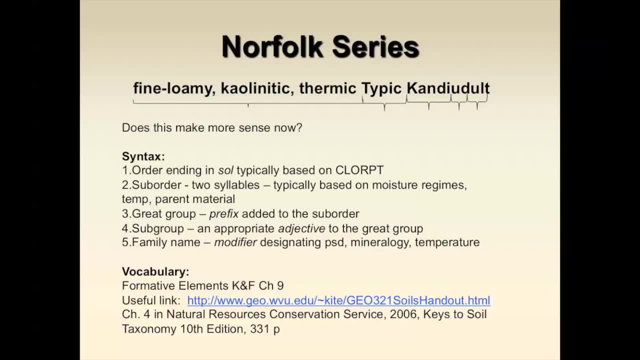 we go. um, we're gonna revisit this again, but your syntax is the alt is your order name. your suborder name is not necessarily two syllables. oh, two syllables. u delta over here. your great group is a prefix added to the suborder. in this case it would be. 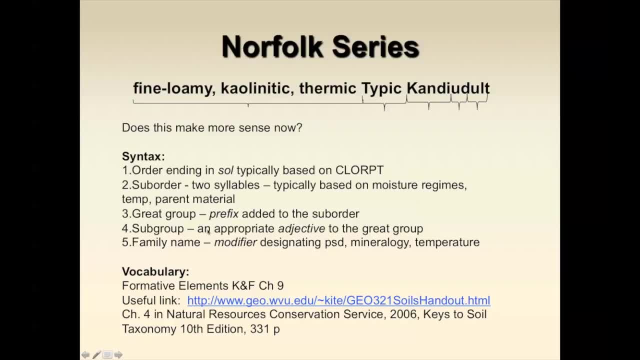 candy. your subgroup is an appropriate adjective, it's typic. uh, your family name is going to be that. uh, modifier, demonstrator, or designating your particle size, distribution, mineralogy, temperature and maybe management regimes. so for your vocabulary over here, so that's your syntax, for your vocabulary, uh, go to conker and franz mayer, chapter nine, or you can. 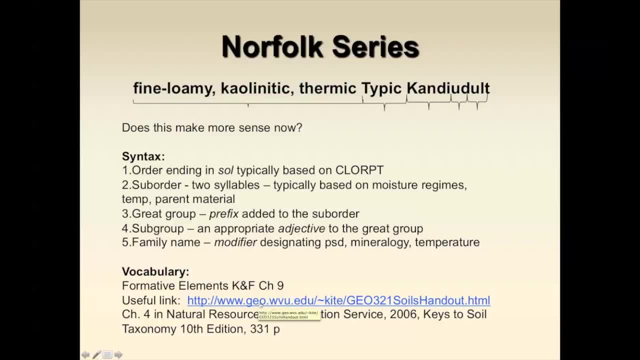 look at this uh link over here as well where you might find- well, you find several hundred, several hundred formative elements. i would say you know usually if you're operating in a particular area, it might be several dozen formative area of elements that you really really would need to know if you were operating in. 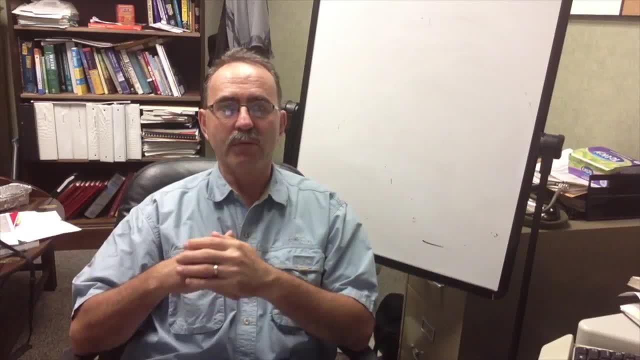 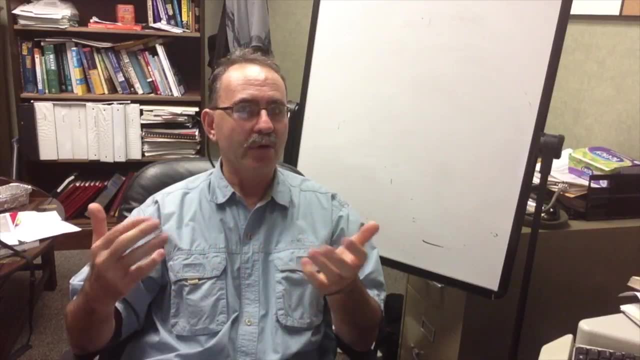 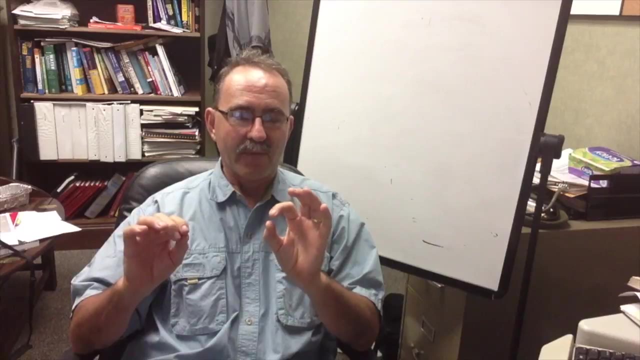 um, in soils. so why would you use soil taxonomy? well, you want to use it to classify soil, but for you you're not going to be. none of you is going to become a pedologist, so probably not. but uh, from that, from understanding that soil, you can. 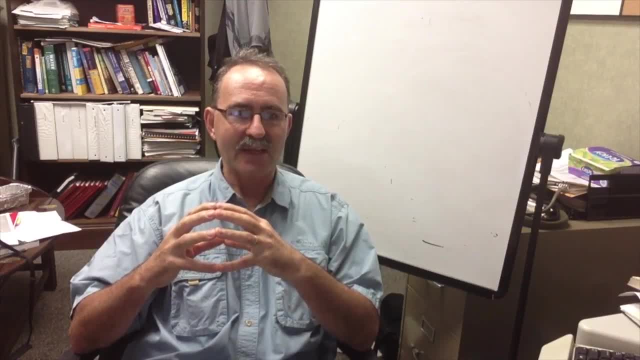 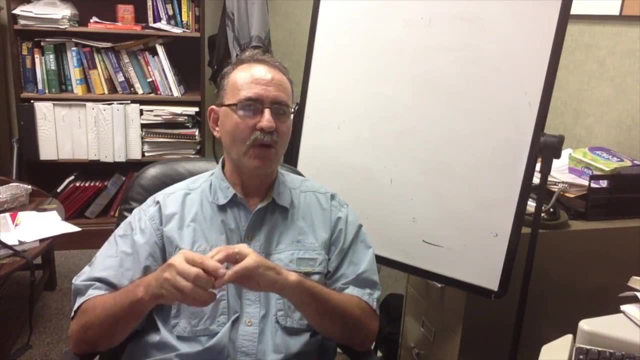 deduce properties of soil and you can use it to classify soil. and you can use it to classify soil properties, that for properties that form a soil based on its classification, and so, without even going to that site, if you're fairly confident that a soil is a fine, typical, fine, loamy, typical, 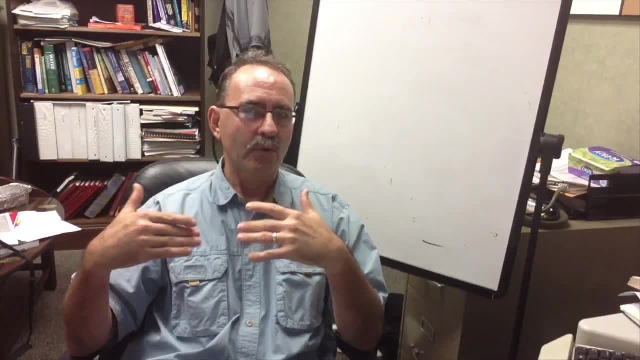 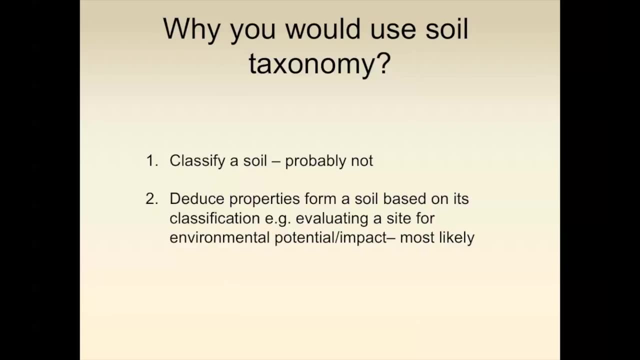 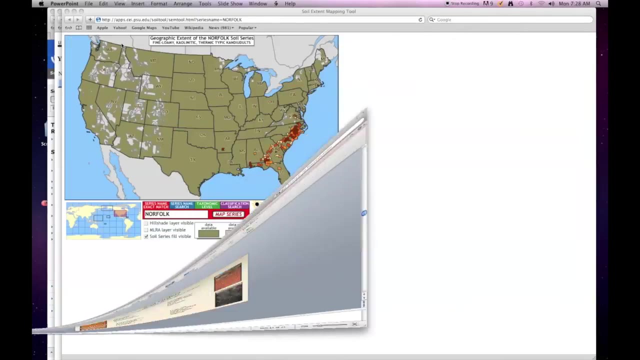 thermic candy, you don't? you you'll know more or less what, what that soil is. um, so soils can kind of be related to one another like kissing cousins. um, i just wanted to maybe just go over here to the official soil description just to kind of give you an idea. um, in the soil series, 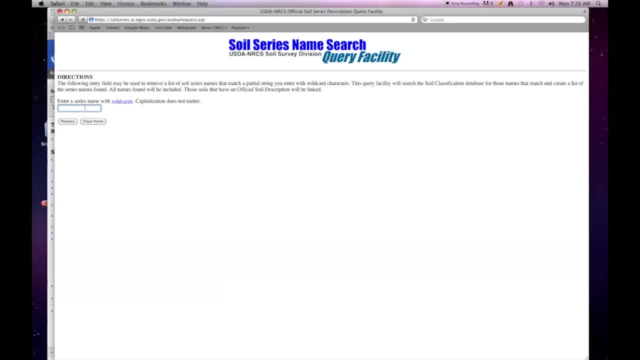 name search, uh. so let's look at, um, say, an- uh, an ailey soil. oh, that's not much good, excuse me. ailey soil is a loamy calinic thermic arenic can haploidult. so if you look at that description, you'll see that this is what the ailey soil might. 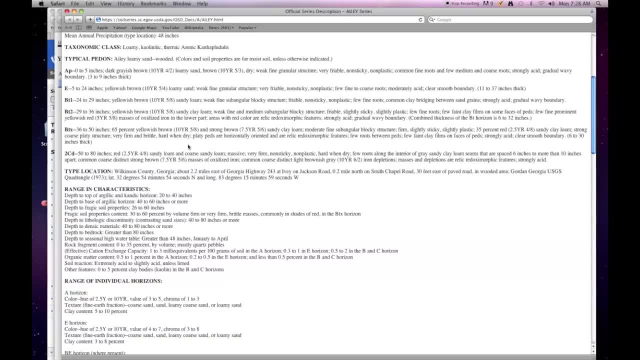 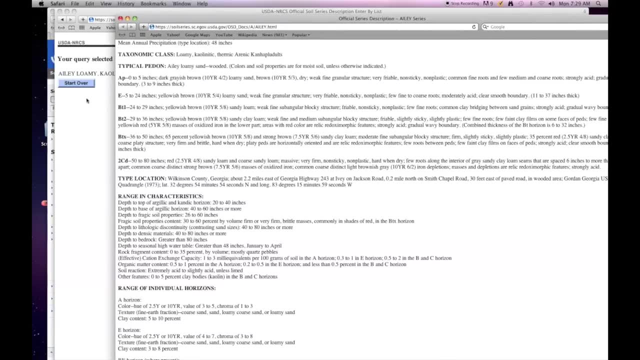 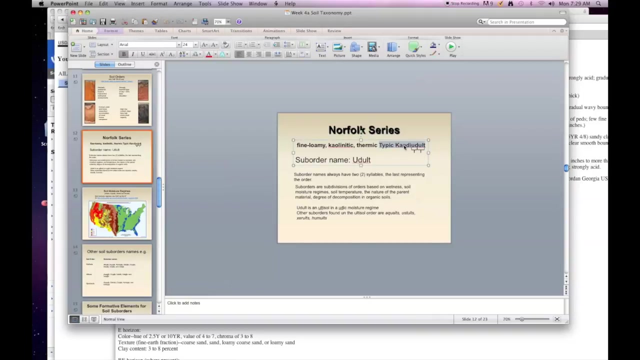 look like. so it's. this is a can haploidult versus a norfolk, which was? or a candy haploidult versus a norfolk. and what was the norfolk soil order? or with a name? let's go back here. uh, the norfolk was a typical candy udelt and the ali is a. 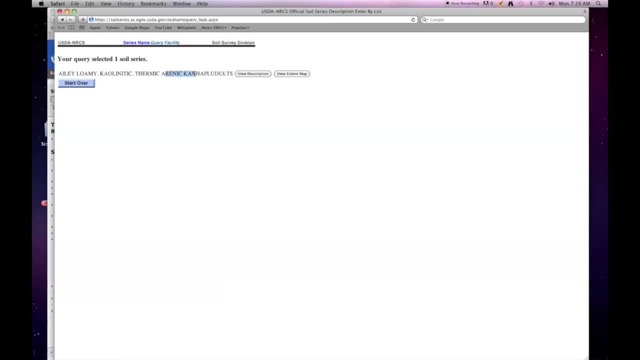 arenic can haploidult, so um, and then you can view those descriptions. I'm trying to think of one other soil order. let's go back here and look at a sisal. sisal is a very common soil order, a soil order that also has various colors to it. but i'm also going to go over toDR portals and you can look at that in the next slide. 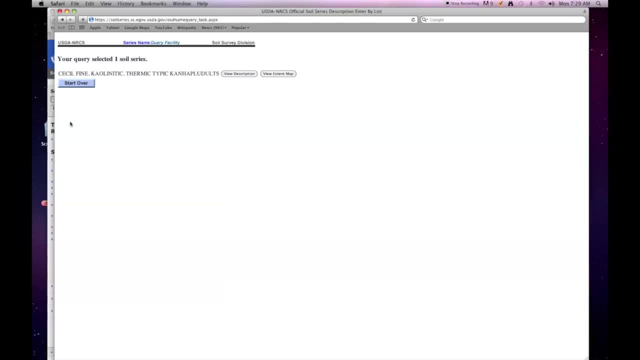 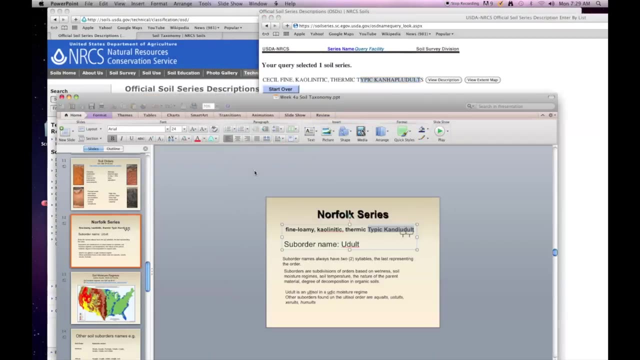 series in the southeast, in the coastal plain. It's a typical Can-Haplodult, as opposed then to the Norfolk which is a thermic, or it's also a typical Can-Haplodult. So the Norfolk and say the Cecil are cousins, although you will never find. not find. the Norfolk, for instance, up in the Piedmont, you'll find it in the coastal plains, whereas the Cecil, you'll find it typically up in the in the Piedmont. Let me do one more here. Rains soil is a wet soil that you'll find in the coastal. 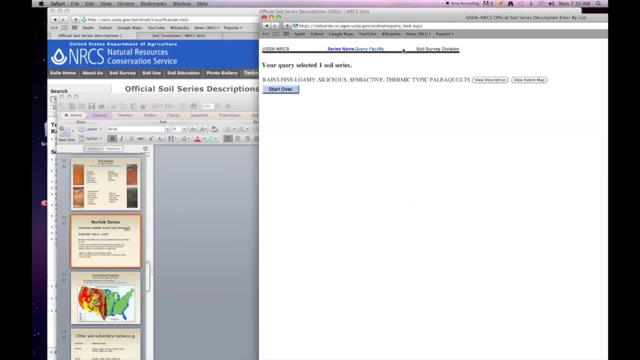 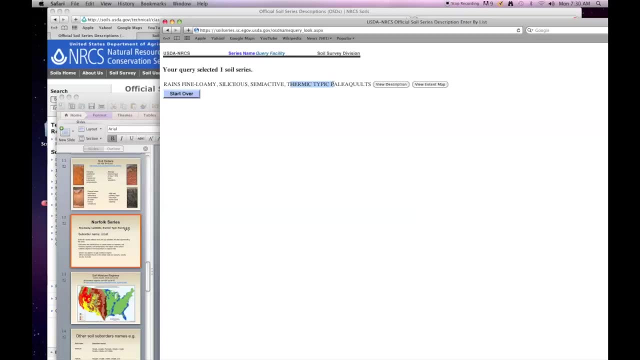 plains, so let's go to the rains- is a fine loamy, siliceous, semi-active thermic-typic paleo-aquilt. Alright, so paleo-aquilt, which would mean it's an older soil, it's an aquilt, which means 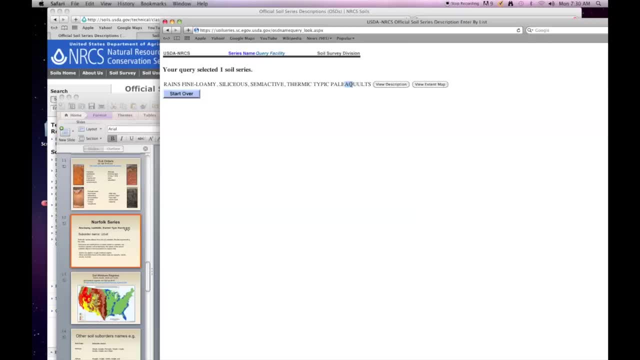 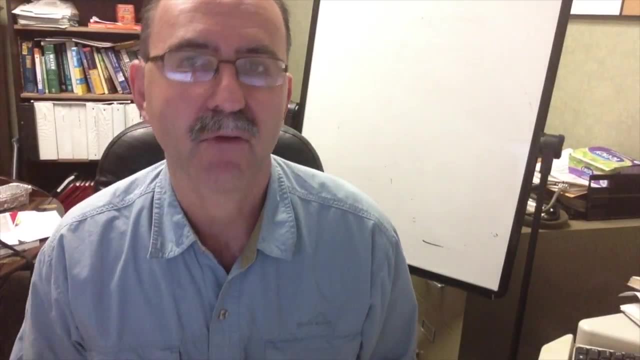 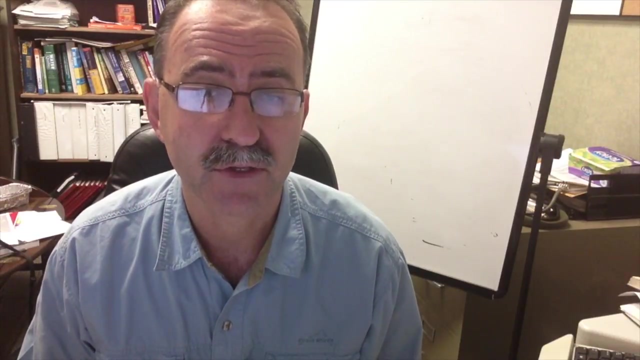 it's got an aqueous component to it, it's wet and of course, it's an altosol. So I hope that that has given you a reasonable idea of soil taxonomy. and well, we'll find out during the exam and I'll also give you some. 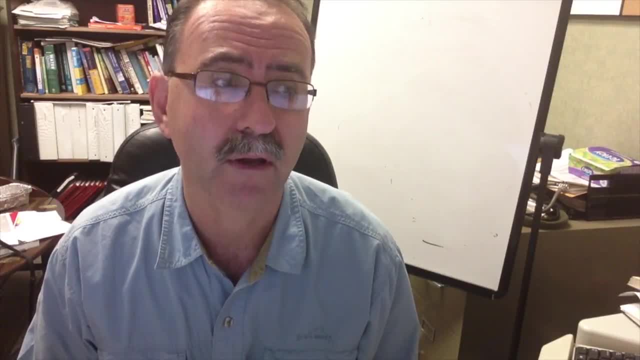 exercises in homework to figure it out. Thank you,